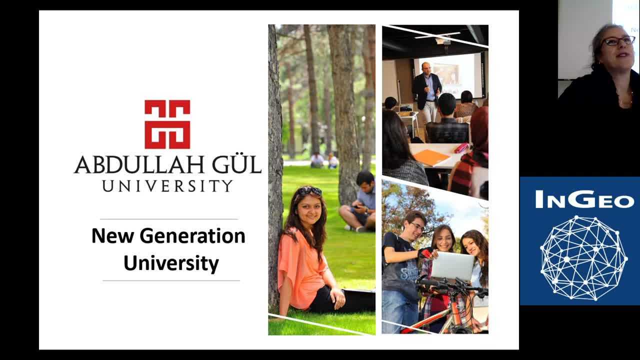 There will be some opportunities for the students. Therefore, I would like to give some brief introduction for our university. So it's called a black university. It is one of the previous presidents of Turkey And he's from Kaiser. That's why he gave his name to the university. 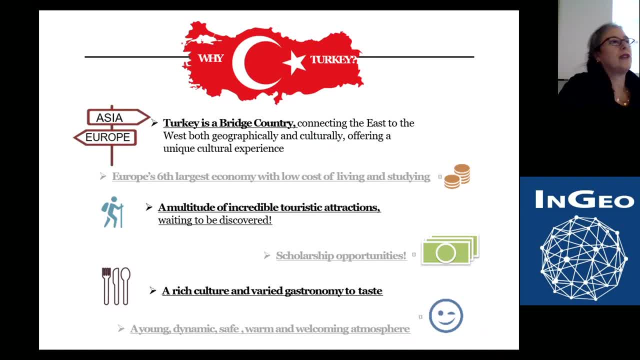 Actually, as you know, Turkey is in between Asia and Europe And we have some touristic attractions and some places. I don't know how many of you have you been to in Turkey, but there are some rich cultures and gastronomy- on some similar topics. 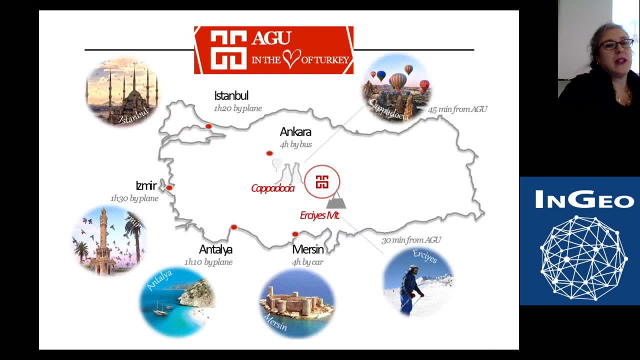 And some similar tests we have. So, in general, when we have a look into the map here, you can see- I don't know if we can follow the mouse, No, From here. Okay, Yeah, So maybe I should take it for the following presentation. 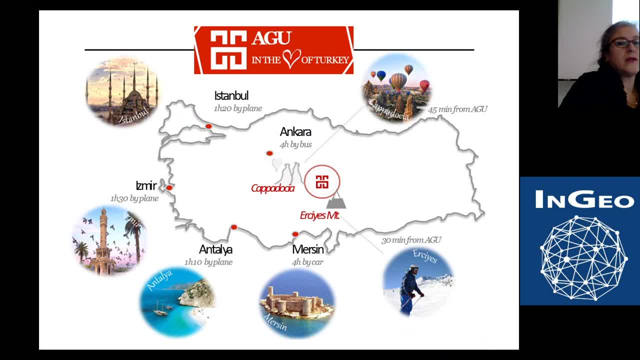 In here. Go ahead. As you can see, we are very closer to the Cappadocia area Which takes place Are just mountain And if you like skiing, we are very closer to that area as a case theory, Okay. 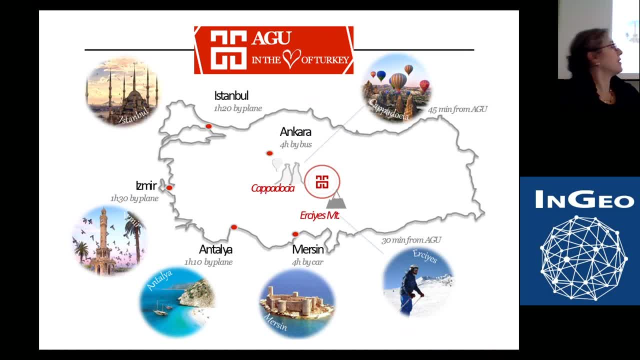 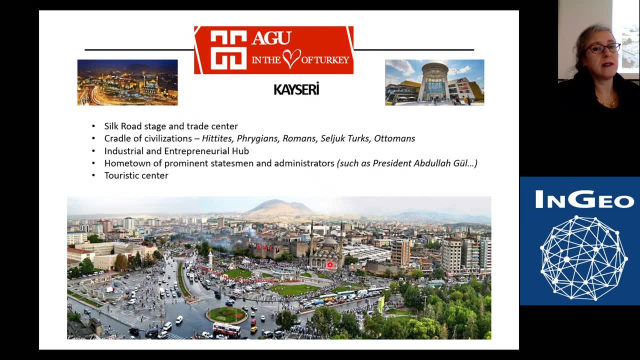 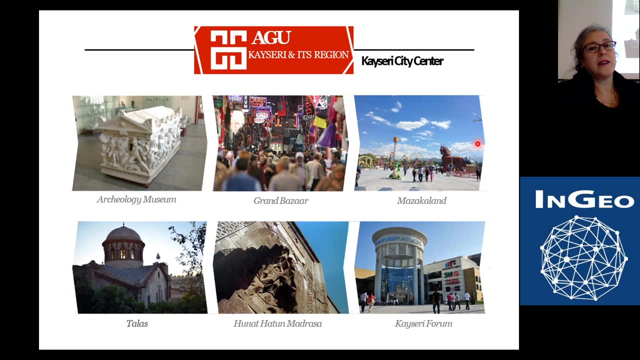 Thank you, And here you can see some important cities from Turkey. It's a stage and trade center within the secret And this is the city center of the area. You can see some historical places and visit And there are some additional interest that you are willing to visit. 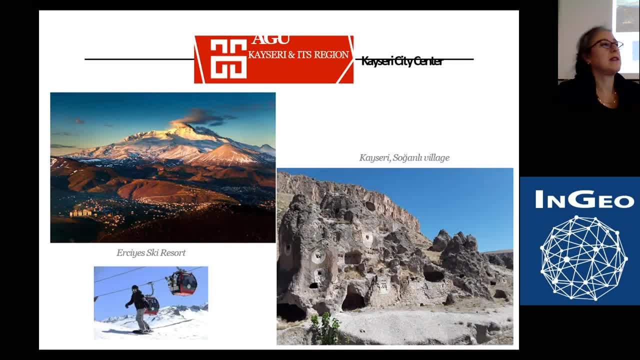 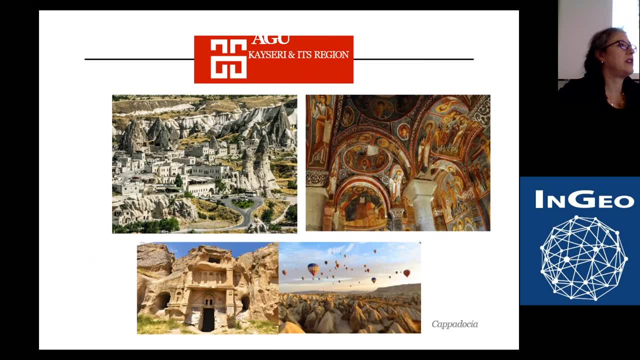 In Kaiser you can have the option And even skiing, And we have some similar places like Cappadocia. But even you can easily reach the Cappadocia region to visit some special places And some special hotels, especially in that region. 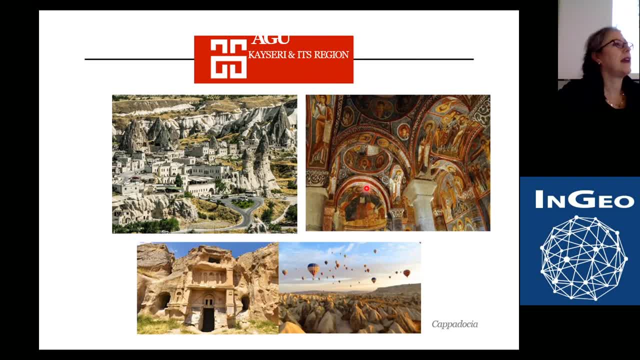 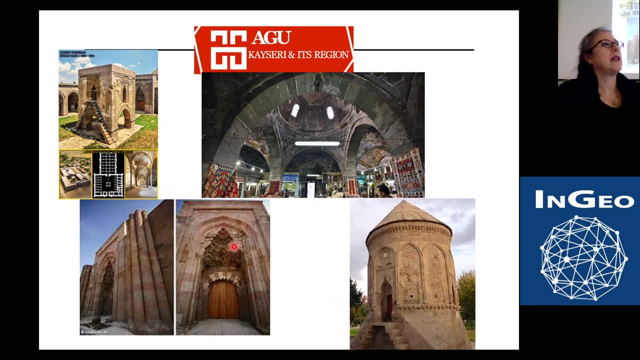 And we have some charts, Very, very ancient and very famous ones actually, And you can have some balloon tours as well In order to see the All around. And for Christy we have some again, Some Ottoman and some such empires. 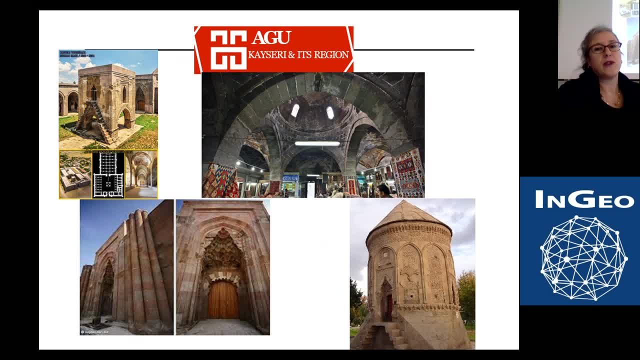 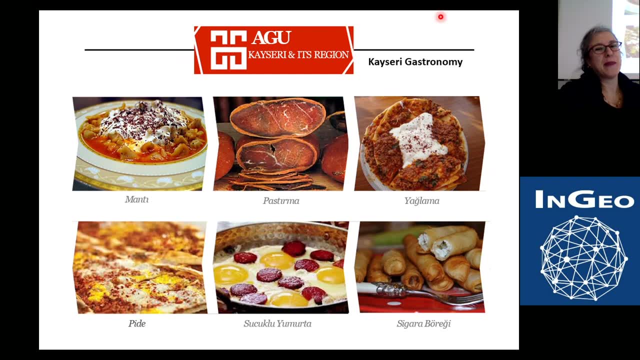 Ancient buildings. If you are willing to visit, you can go there, And the important point would be the gastronomy. Everybody likes that And we have some special taste Including some kind of special meat You can also easily have. And then it's very famous, especially Kaiser with the. 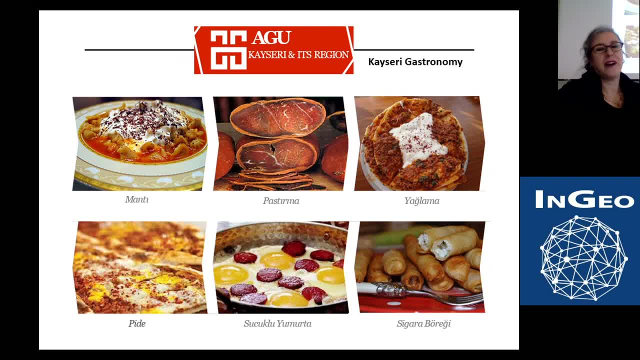 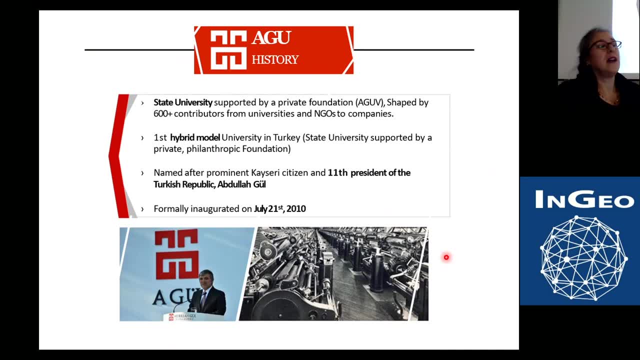 Which is called pasta. It's a kind of dried meat that we are having too much, Or probably you will love it. So for our university- As I told you, it's the one of the previous president- we have- And actually we have- a story of our building. 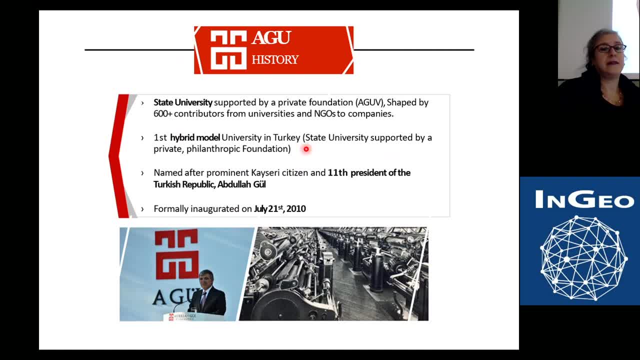 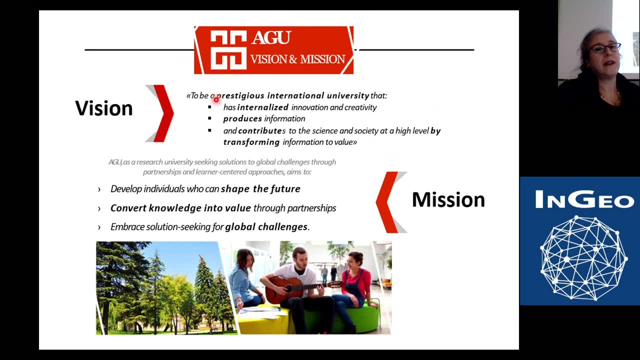 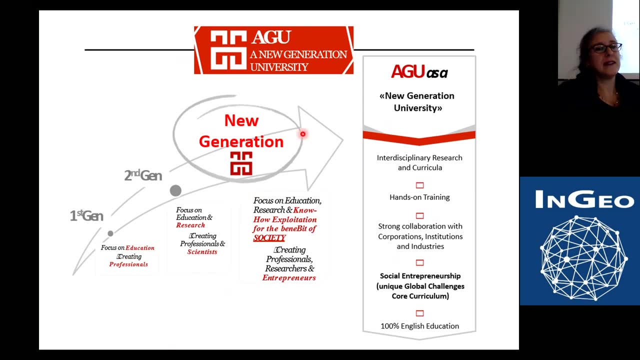 Because we have renovated the factory. That's why it's really worth it to. I would like to share an over to the photos, So we have some visions and missions According to our university. if I am Going a little bit faster, 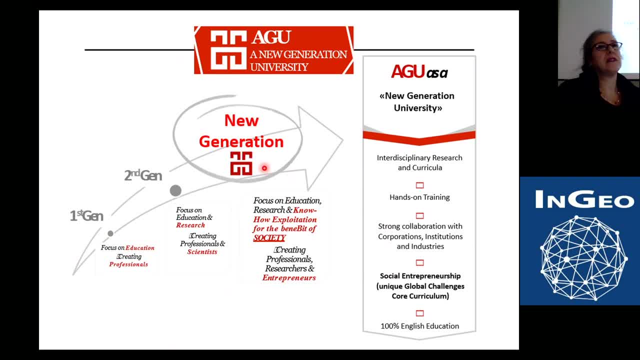 It's the kind of new generation university We are actually dealing with some interdisciplinary program And we are actually considering in connection between the Different disciplines And a hundred percentage English education We are having for all the departments that I have to also mesh. 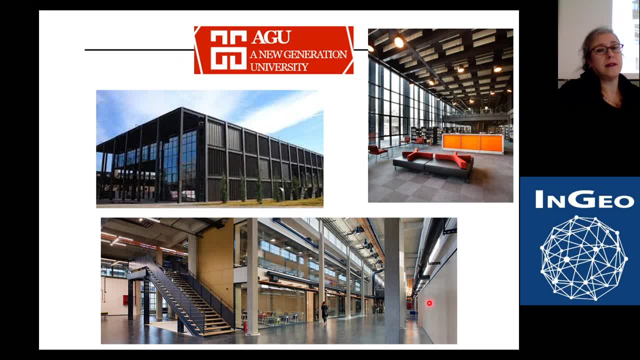 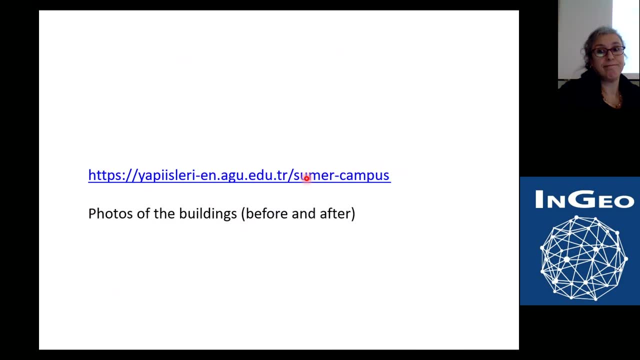 And then we have Some of the buildings And here you can see Some of the buildings and It is actually There's a price that That had because of the renovation of the steel building. This is our main and rectory building. 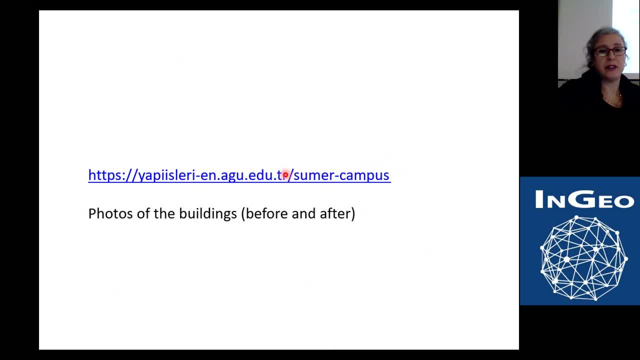 And let me share some of the Campus photos, but I don't know if I can open it Because of the pointer or the other stage. Here You will see, Because architects Really worked on that area In order to actually 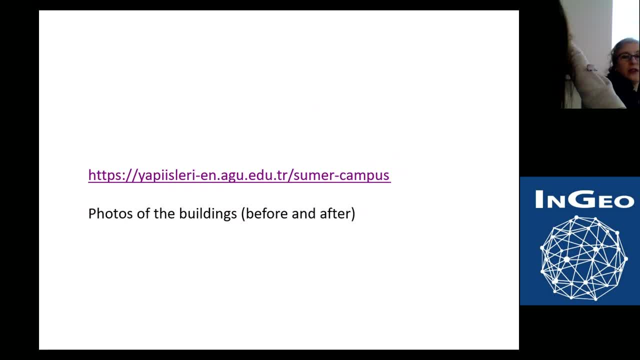 Keep the preserve, the area Which is really ancient and important for us. I don't know if you can reach this. Yes, And in our campus, as you can see, This is the big image. No, I'm going to go out from the presentation. 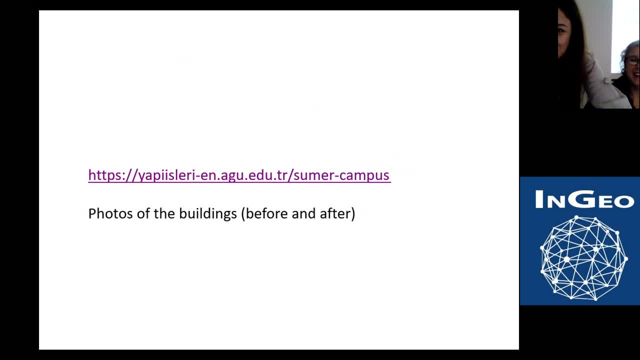 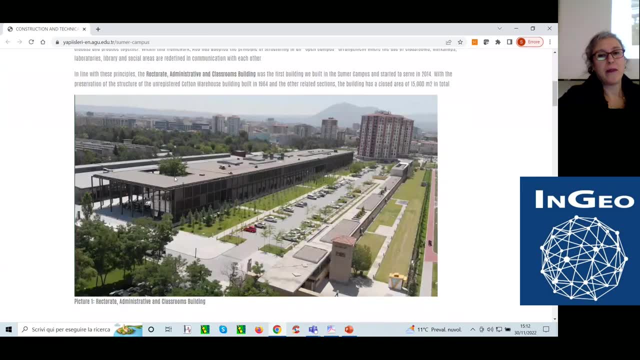 I'm sorry, I don't know how to do that, But I'm going to do it. No, don't worry. No, Okay, So now I should do it. Let's see. Yeah, Okay, Okay, Here you can see our. 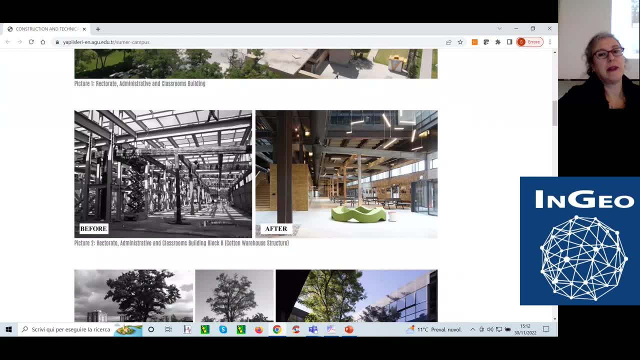 Building within the main campus. It's a Good place And I would like to share the Main building. That's Was earlier As before, And then after renovation. we have some places, especially for students Or for the people who like to be there, or we are actually. 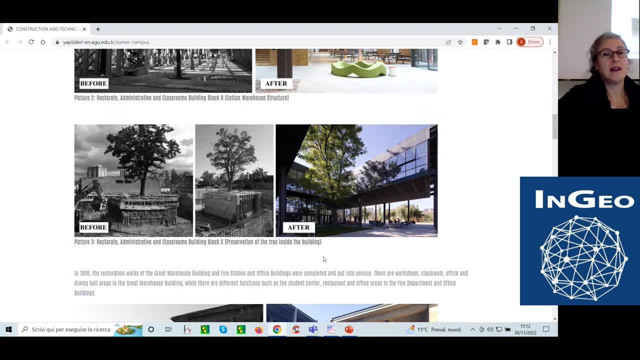 Preserving some trees, some special trees, And then, in order to have this, Let's say, structure, And we have also keep some of the Previous. They are all Warehouse And we are now having classroom buildings inside the offices and et cetera. 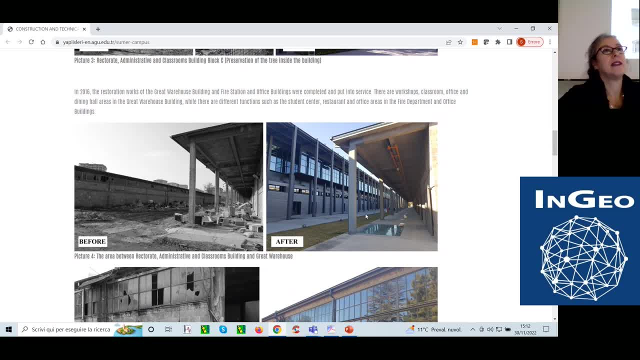 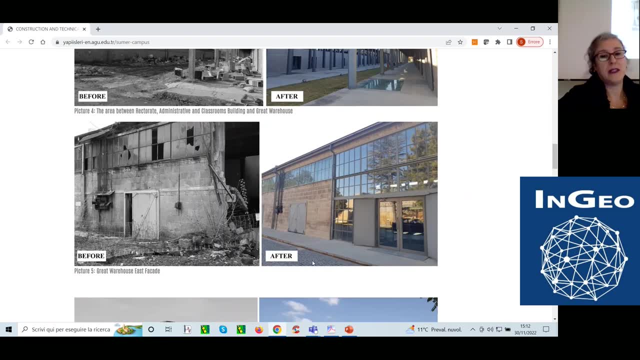 And here you can see The renovated part of the Facet And before and after. Now we are actually Reusing And then, Yeah, There is a sustainable version of our campus. We can say: this is the Fire. 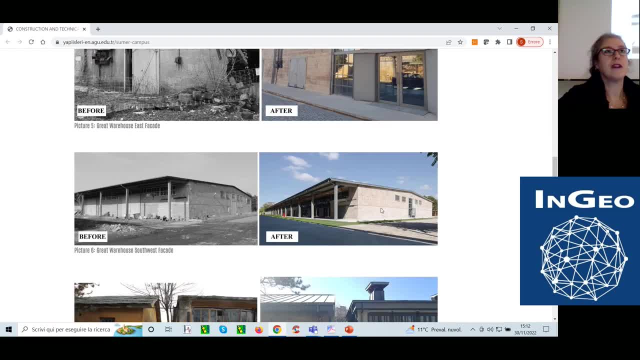 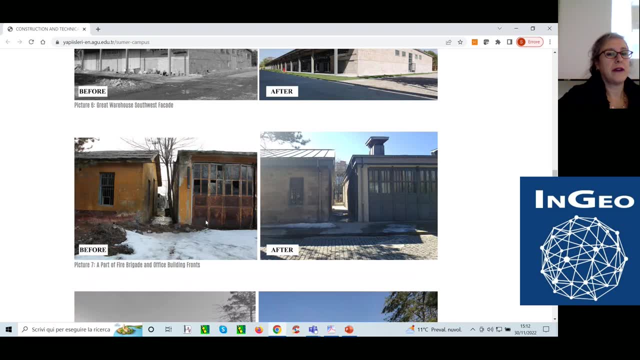 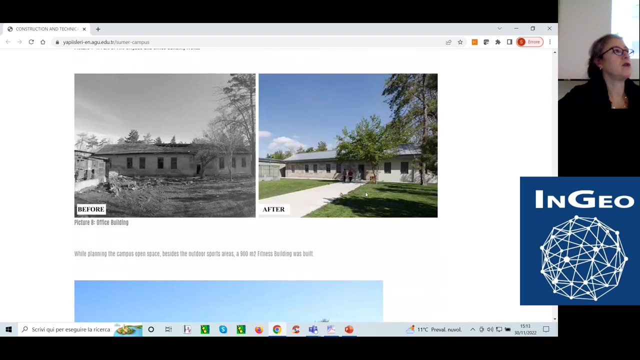 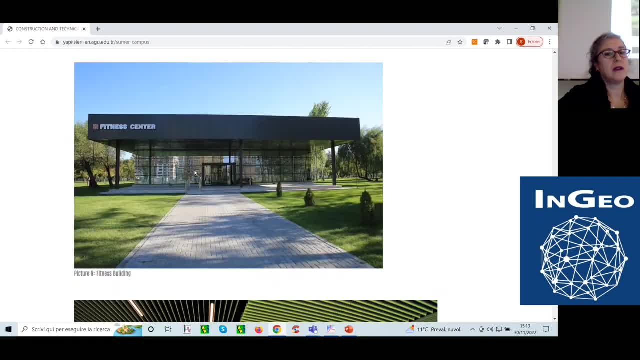 Innovation in that region. and then, yeah, We are also still using as an office In here. for instance, I know we have newly eh constructed some Buildings Like fitness centers and some laboratory Buildings And, as you can see now, 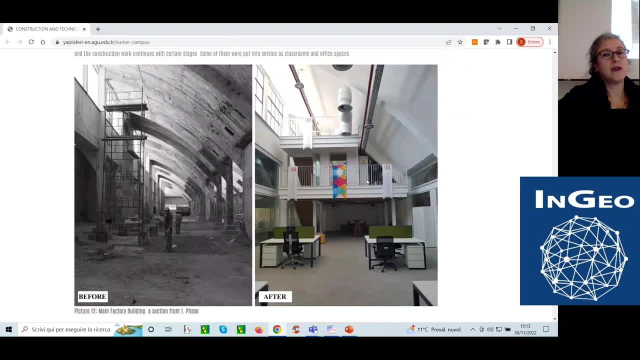 Yes, We are Actually dealing with This Factory. This is the main Factory building, And now they are all Covering the columns With some Geotextile Material in order to again Reinforce The building. 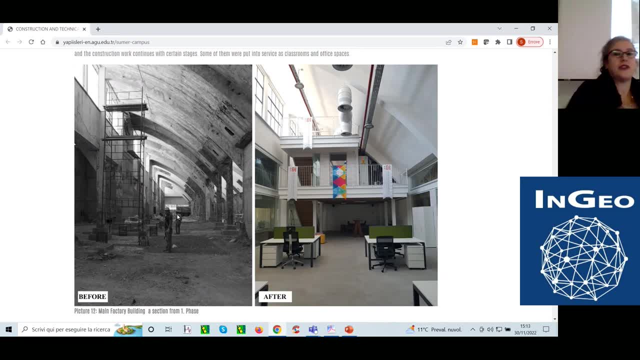 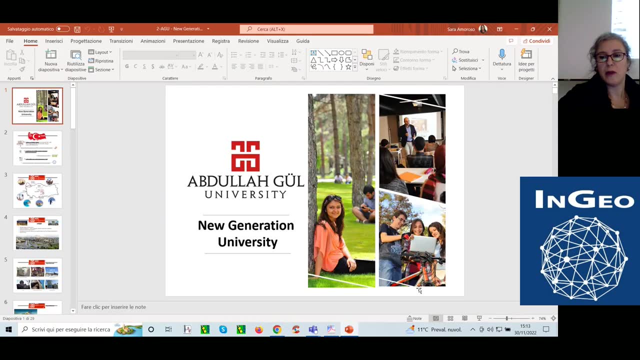 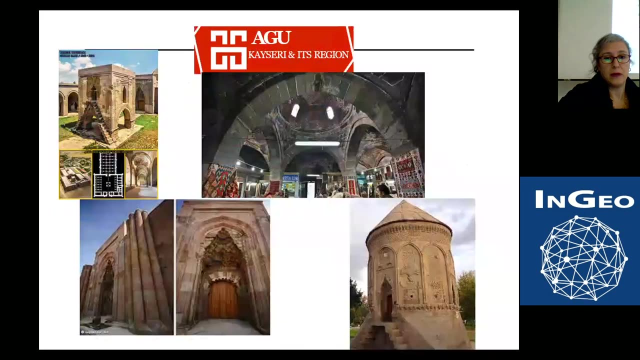 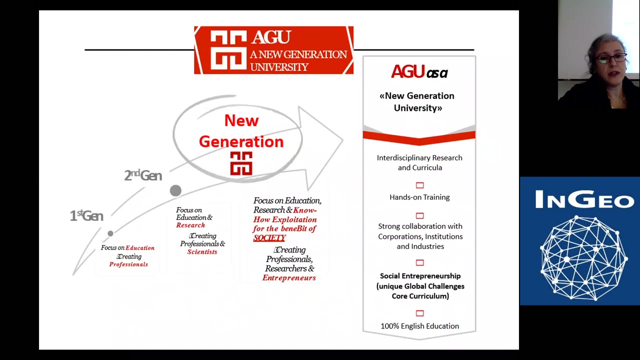 And uh, or the structure. maybe we should say that. So after giving this information, I have to return to my presentation. Hopefully I can reach my page. So, with the numbers that I have to say in general, we have a limited number. 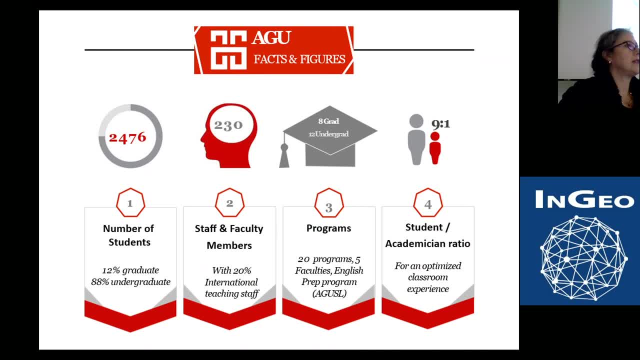 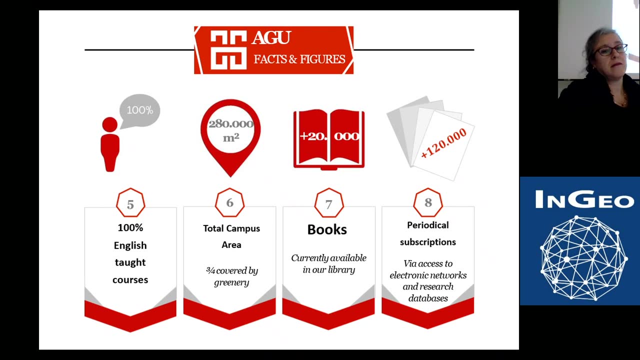 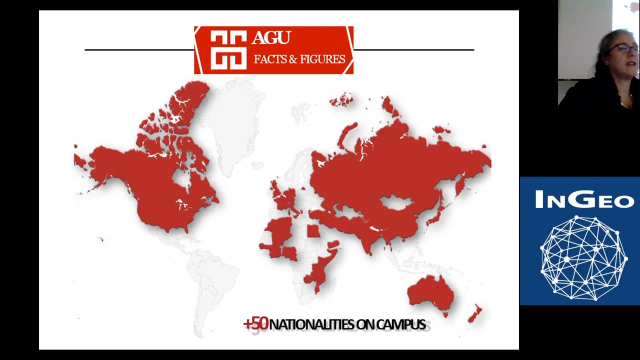 which is called kind of a basic university. I don't know how staff member or faculty member you have, but it's a very limited one And we have 20 programs and with the five faculties, including 100 percentage English taught courses And you can see different nationalities. 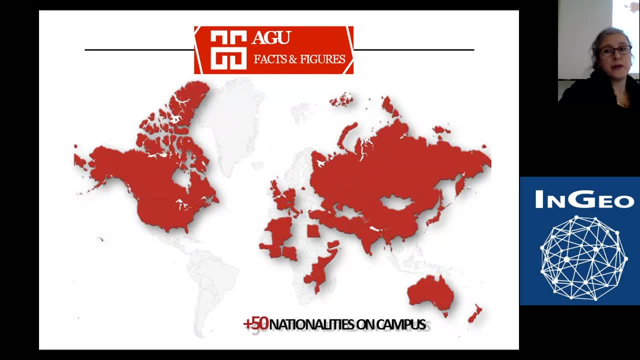 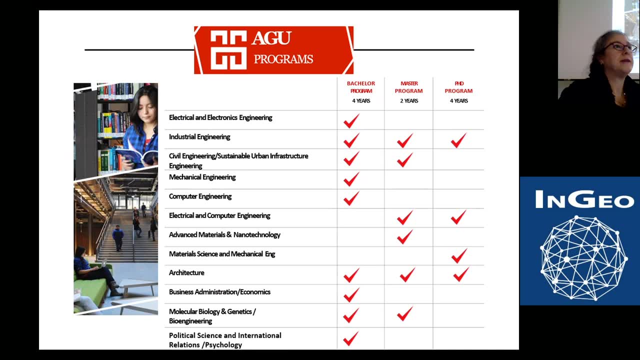 We have even from Italy in our campus And here you can see our departments. These are the actually departments that we are having so far And we are not planning to open any medicine or medical faculties Depending on the technical issue. we are all focusing on that. 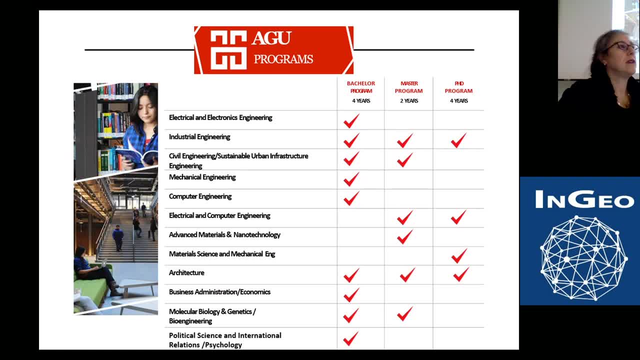 And from our civil engineering department, we are limited staff in there And then we don't have any master program. We have a different master program. We have sustainable urban infrastructure engineering, which combines all of the again urban planners or other disciplines in order to have a program. 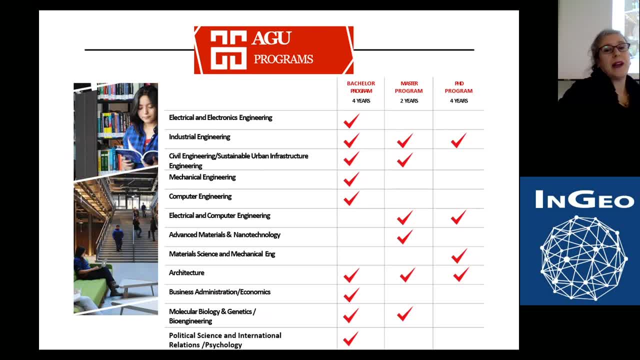 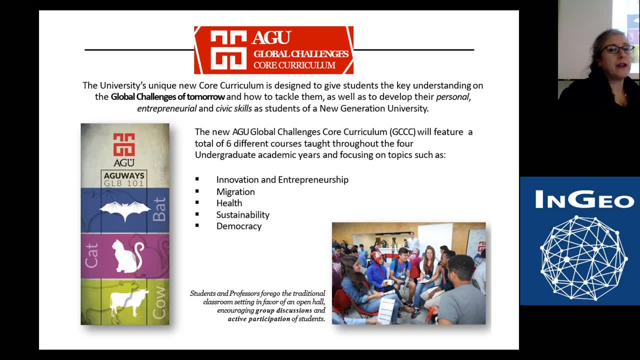 Especially- there are some examples in UK similar to that And here you can see the other- actually programs that we are having, And we are actually having some global challenges. We have some special lessons, including global challenge GLB courses. All students are mandatory to take these courses in three years period of time in order to have an idea about some entrepreneurship, or even with the sustainability part. 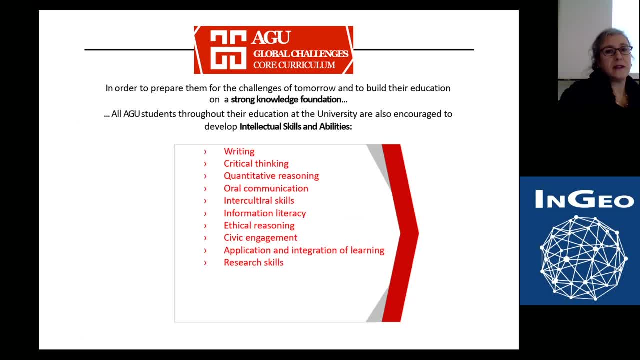 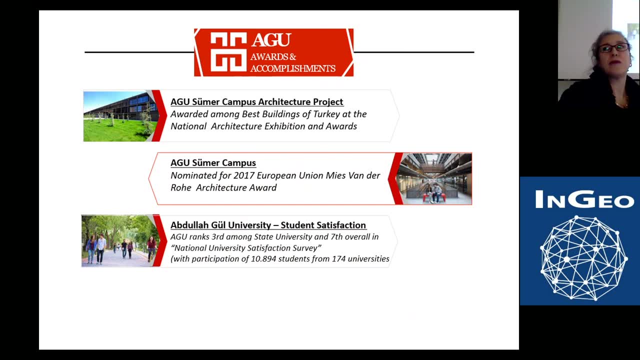 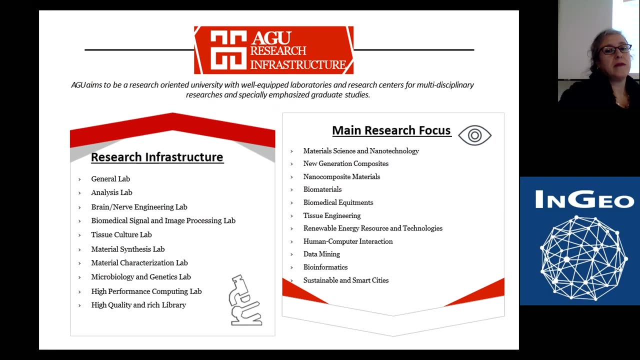 And the other things is really critical depending on GLB core curriculum. we have And we are having some especially for student satisfaction. They are really like our university And we have some research centers And mainly we are focusing on especially for the bioengineering part, like new materials, biomaterials and et cetera. 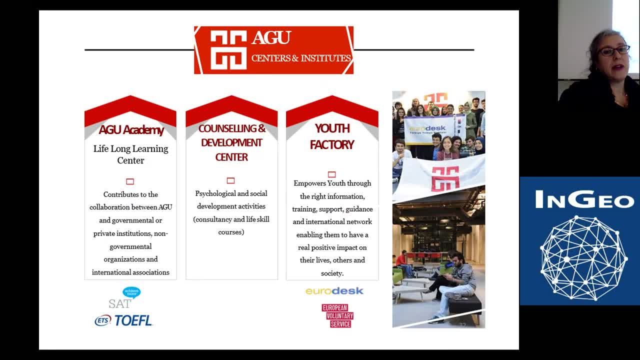 I should also add them to you. And we have additional places like youth factory, which also supports the students especially for their needs or for their additional things. It's a kind of new Maybe term for all students for us, And here you can see some of the examples from our dormitories. 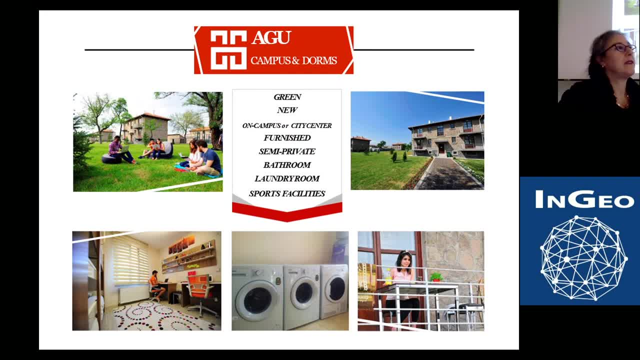 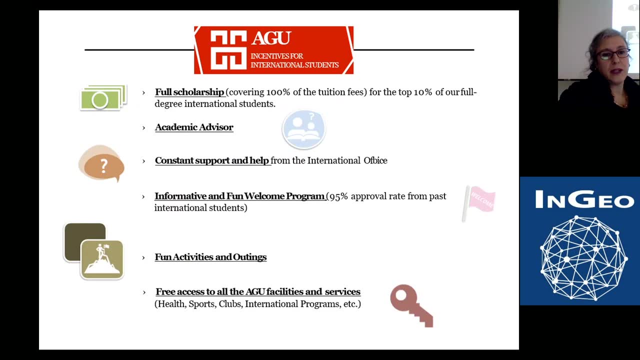 These are also new. They furnished, but they were the places who sit, the people who worked in the factory, as before. Nowadays they are using as a dormitory. So, yeah, there are some additional activities that I might say, And we have some partners actually, 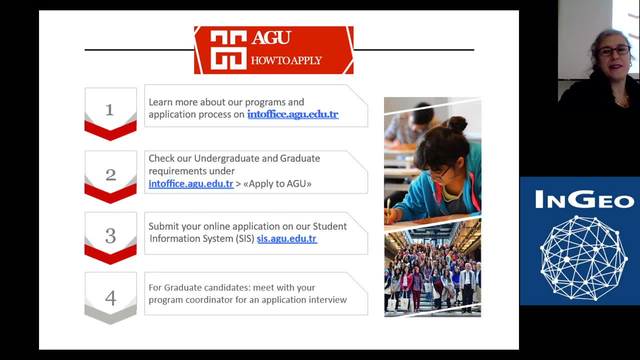 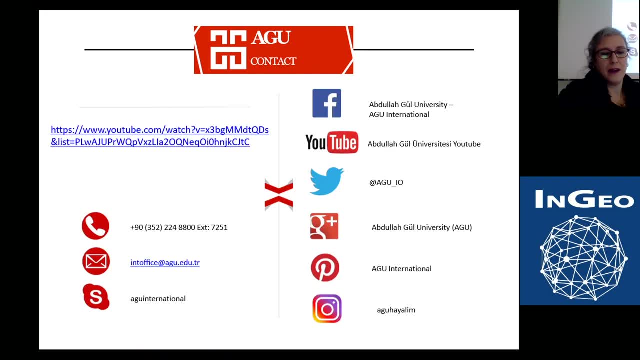 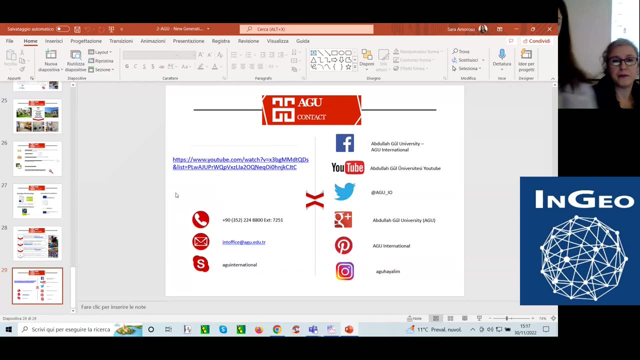 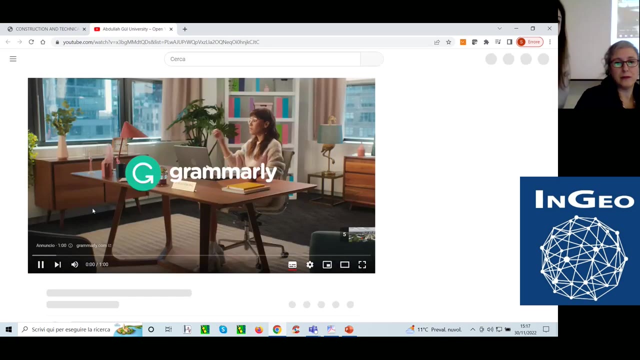 And you are one of the partner, And I would like to share just a short video for our showing University, but probably I need to change it. It's a very short video I would like to share with you. I have almost a few seconds. 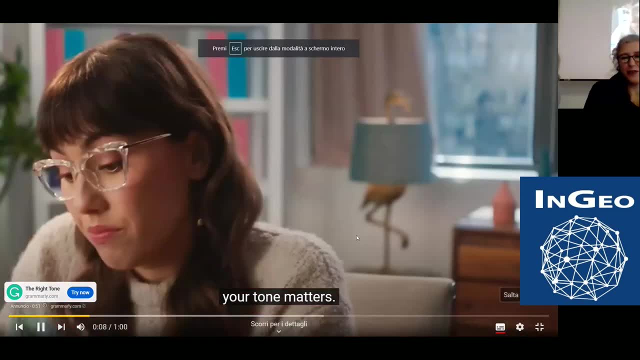 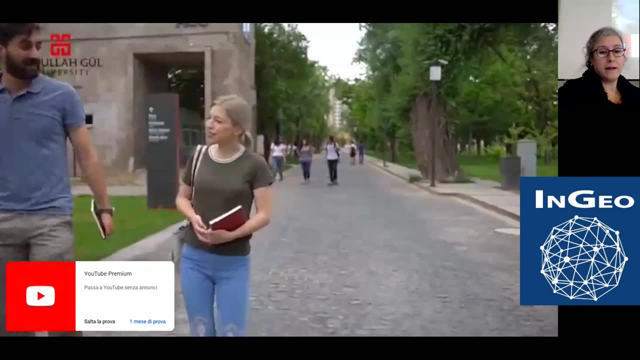 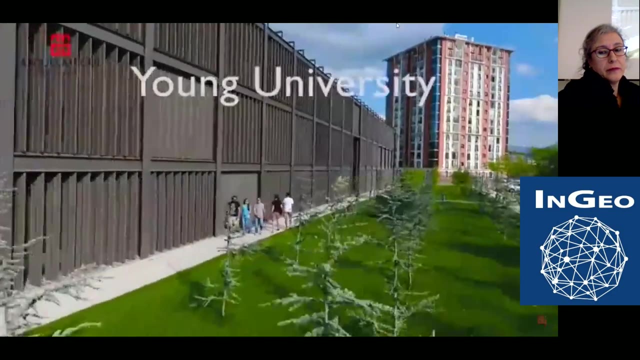 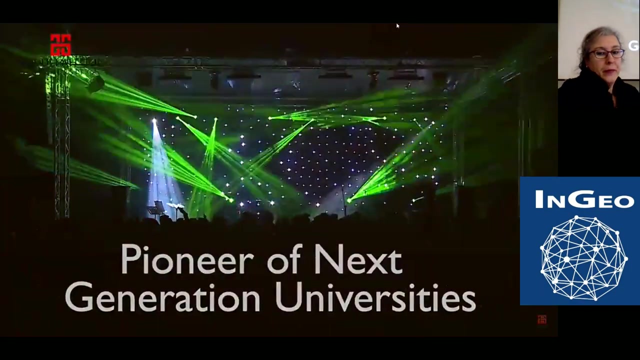 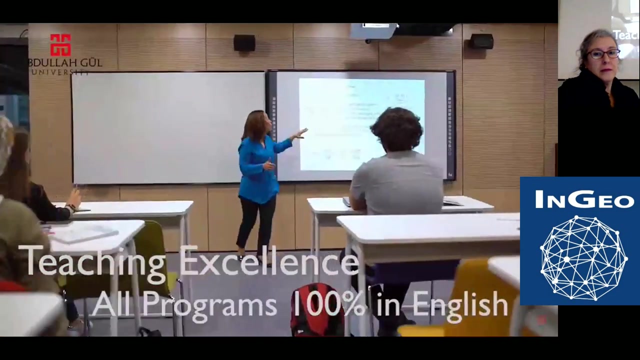 Okay, Can you screen? Okay, So I'm going to go to the next slide. So that's it. If you have questions, please, or comments, you can comment on the slide And I will be happy to answer them. 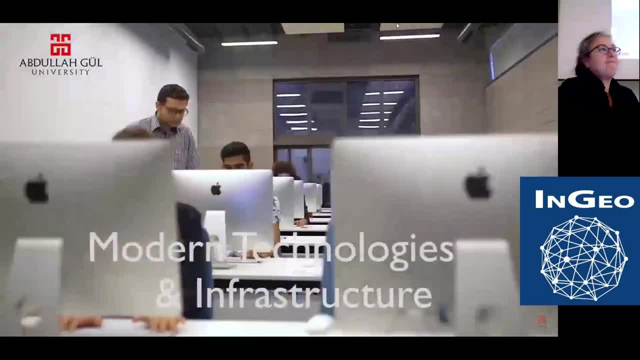 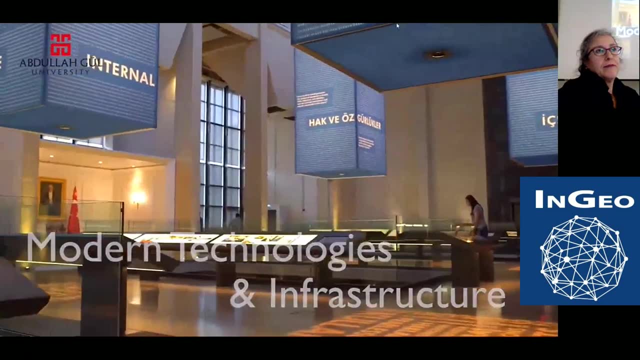 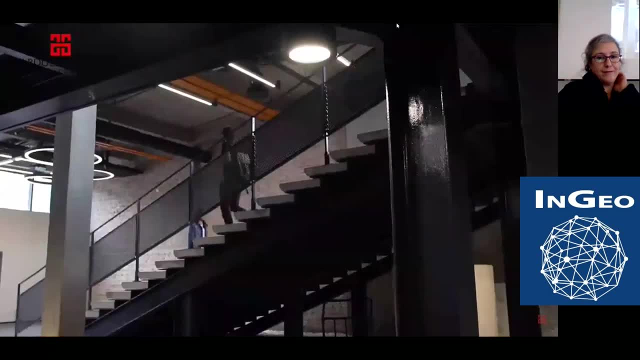 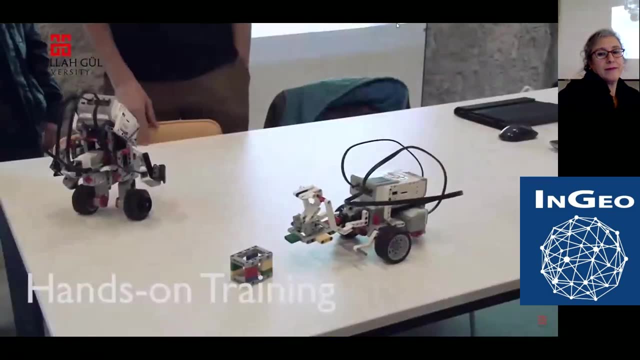 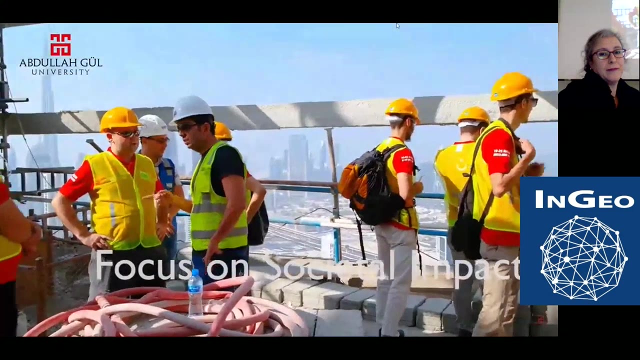 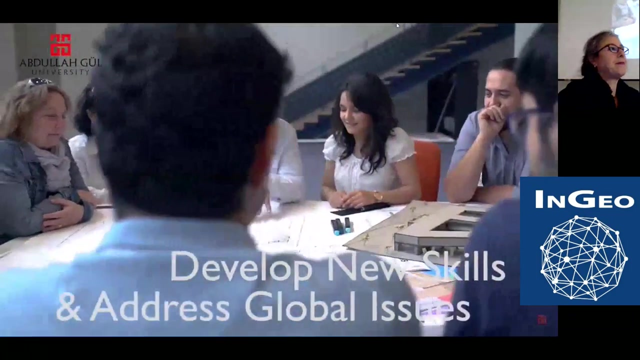 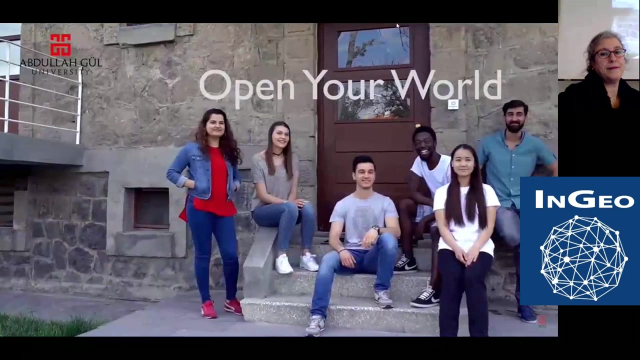 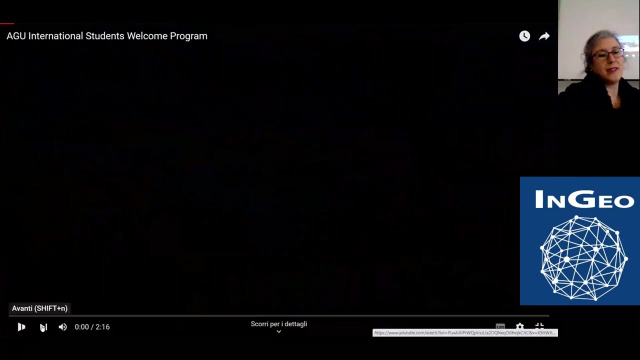 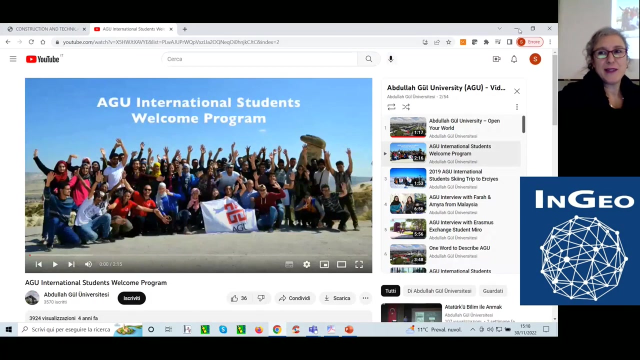 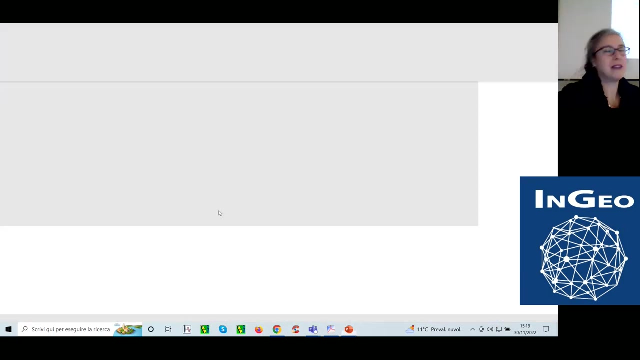 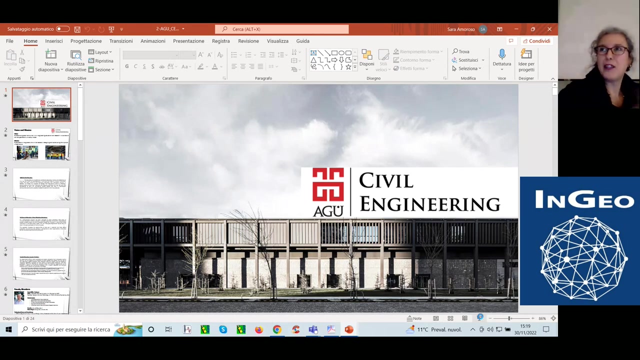 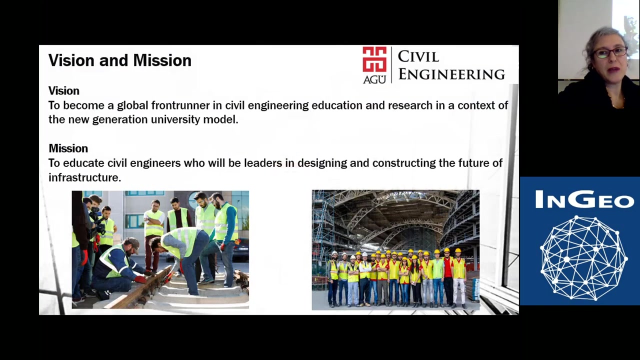 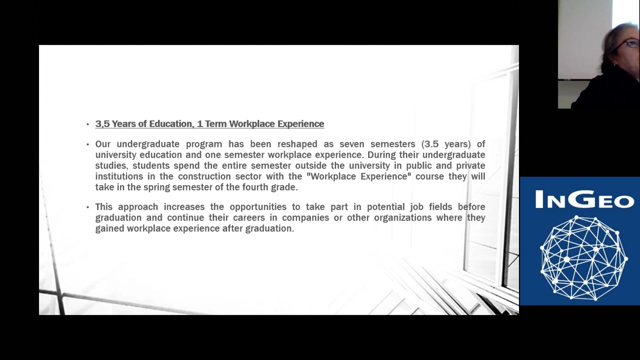 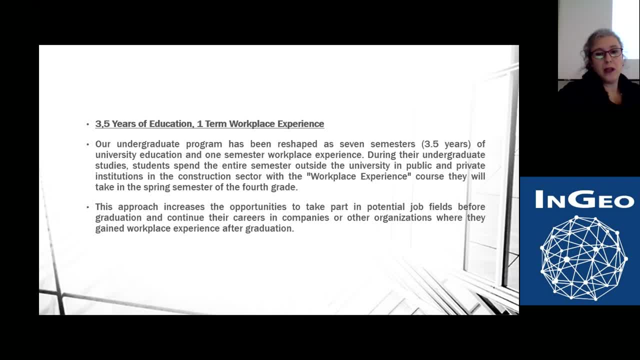 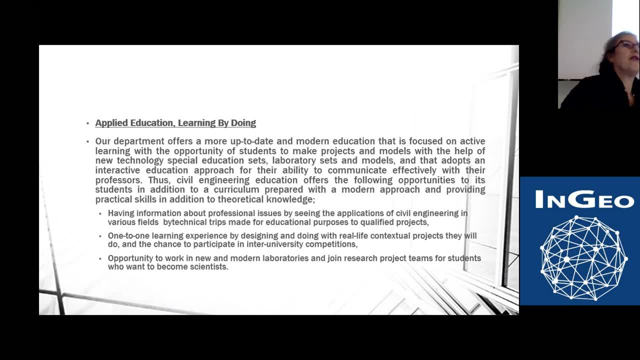 So that would be the good opportunity for them And what else we are having. We are actually considering applied education. We are focusing on you should play and learn. How can you do that? It's making some models, or having some special apparatus in order for you to have to make your models. We are really considering that. 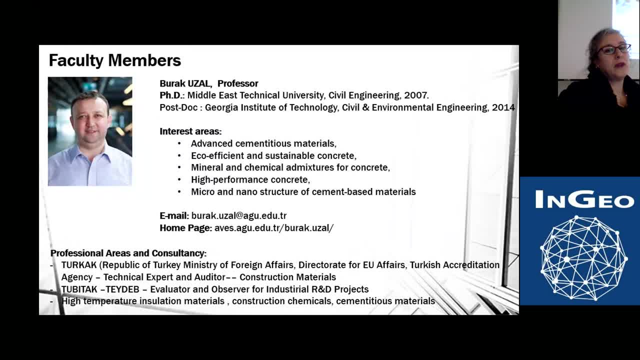 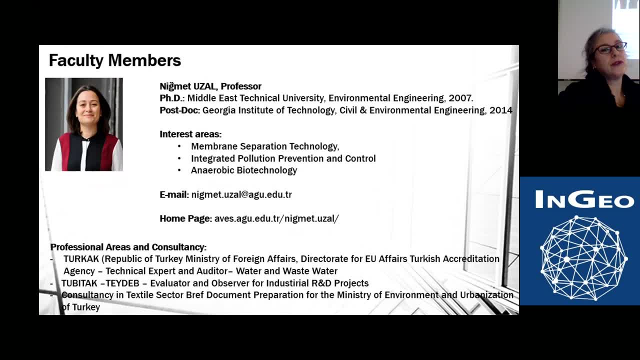 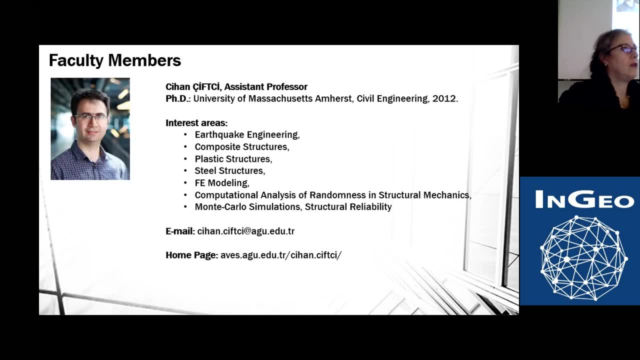 And we have some limited professors. Burak Hoca is dealing With material science, for instance. Nimet Hoca is working on the sustainable issue and other stuff Also deals with the earthquake engineering and structural dynamics in somehow, And he's also having a project regarding to the wind turbines. Actually, now he's working on the material that they are dealing with. 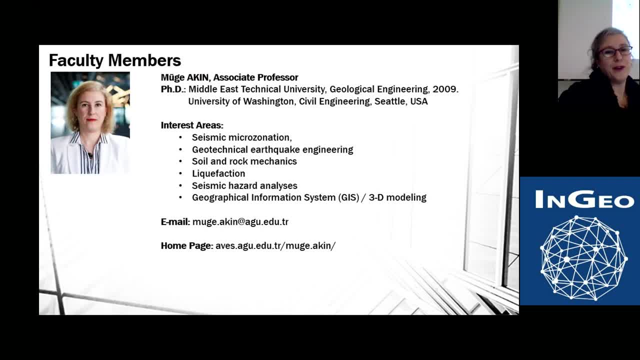 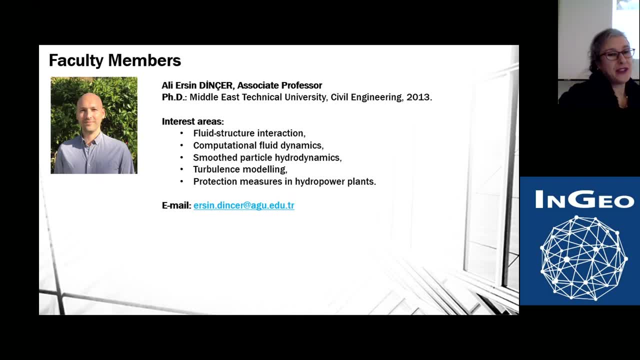 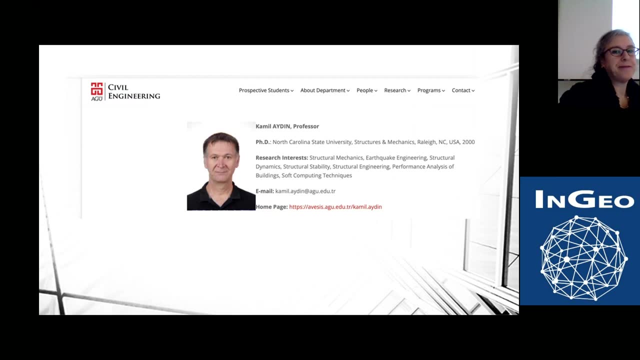 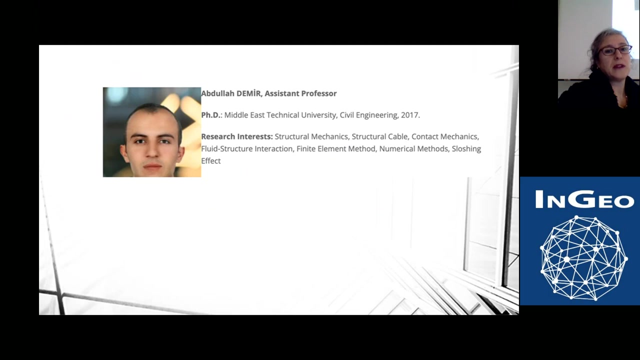 And you know- I hope you know me And the other stuff from hydrology. hydrology he's dealing with the fluid structure interaction especially. we have another professor- I have also met with him in Pavia- I have been to Pavia, by the way- and he's now working in the engineering and structural mechanics- and another professor from structural mechanics part and with the railway transport. 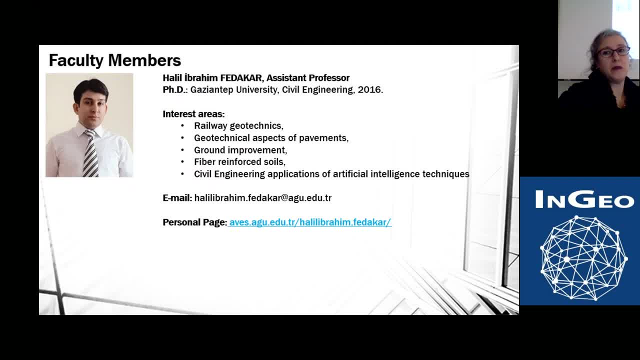 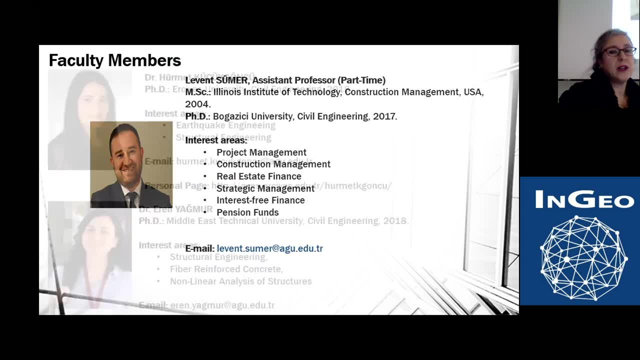 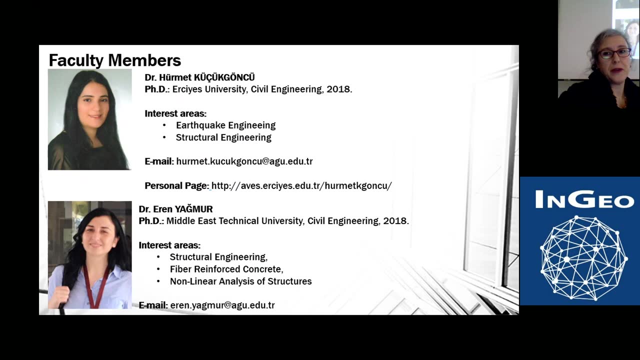 And the geotechnics. there's another colleague that I have highly And we have some part time faculty members for project management and et cetera. and these are the faculty members. They're also dealing with generally earthquake engineering and structural engineering. 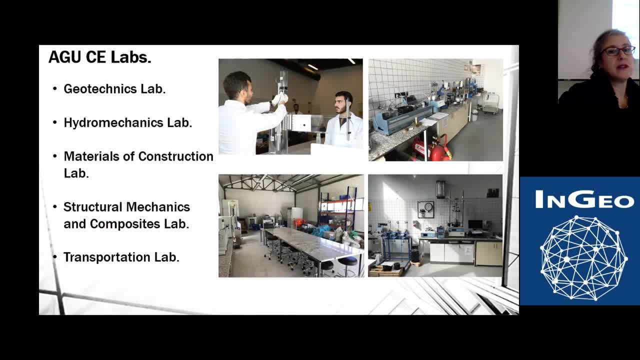 We have some laboratory conditions for geotechnics, for hydromechanics, material of construction, structural and transportation maps. We have new equipment But unfortunately, as I told Professor Amaroso, we don't have any technician. Therefore, we need to have and improve some of the things by the help of him or her. 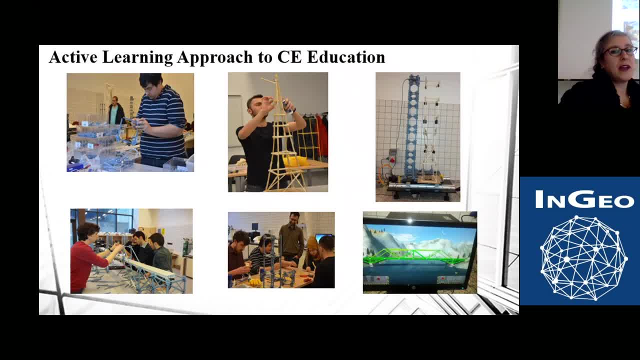 And for the active learning. as you can see, we have some special Legos- I don't know if you heard about it, Pasco, which is named- and you have the pins and then you can make your model, having this experiment And then with a shaking table. 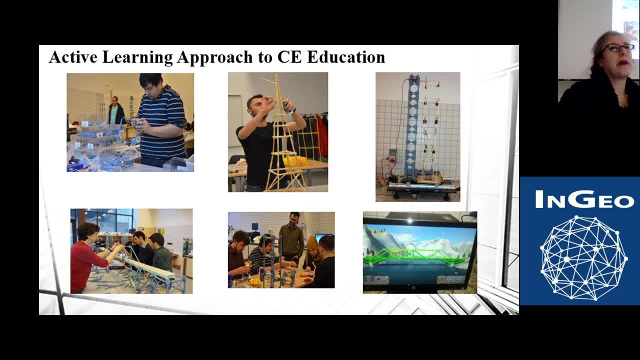 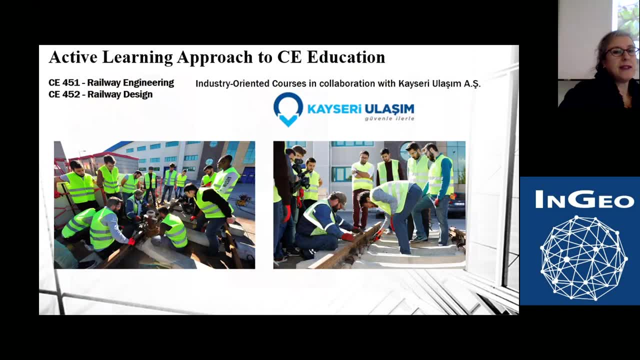 You can understand the structural behavior, or even you can prepare a bridge and then you can apply some train or car load, et cetera. And even they are going for railway engineering and railway design in order to learn the states for how it occurs for the railway states. 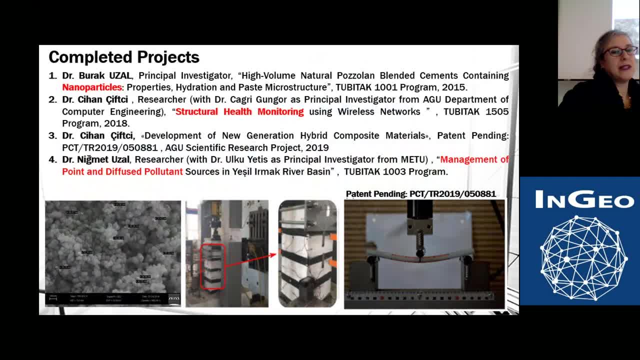 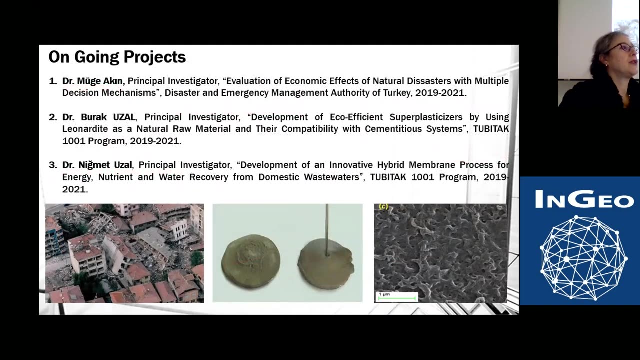 And you can see some of the examples for completing at that stage, but I have forgot to update some of it. But For the structural health monitoring or some material science, you can find different options and different projects that we have already completed And I was also involving a project which is related with the economic effects of the natural hazards related with disaster and emergency management authority. 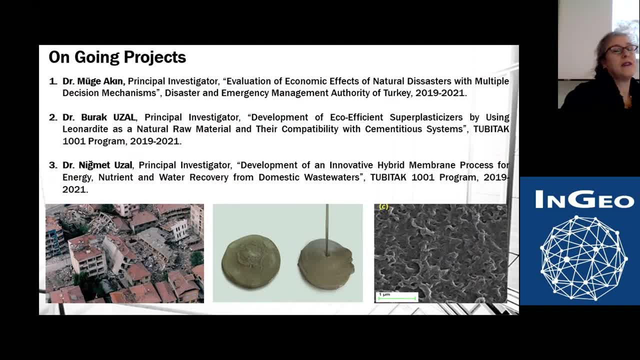 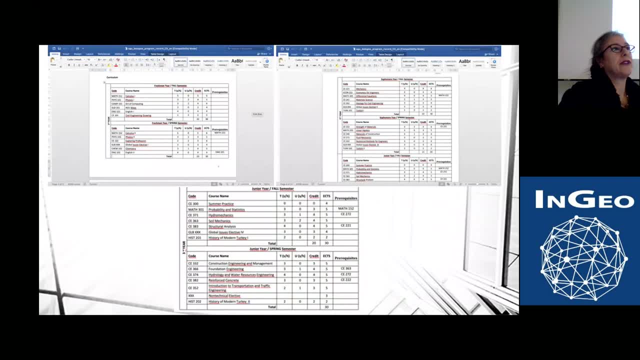 I have completed that, but it's also another area that maybe we should also discuss about, And for our project And for our case, we have some undergrad courses. If you are willing to interest, I can give the more details of it. 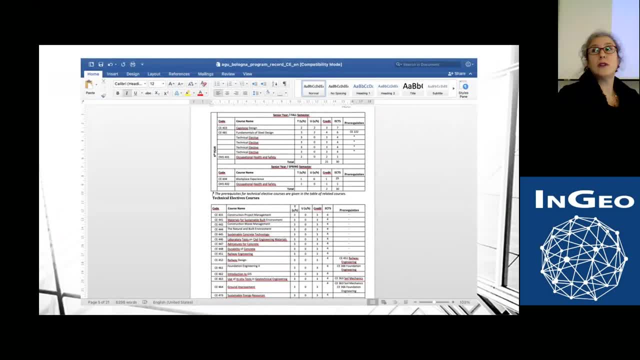 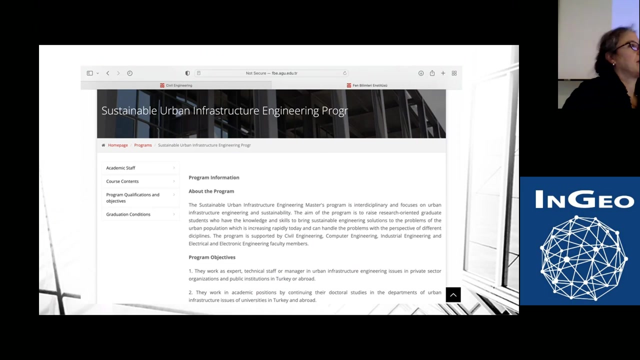 And there are some options, especially for The Technical courses. did I do anything wrong? No, no, Should I piss? Yeah, I'm always working, Yeah, Okay. So for the program sustainable urban infrastructure, I can give again brief information after the maybe presentation. 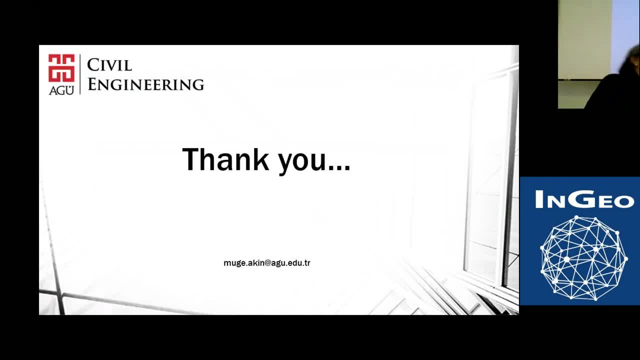 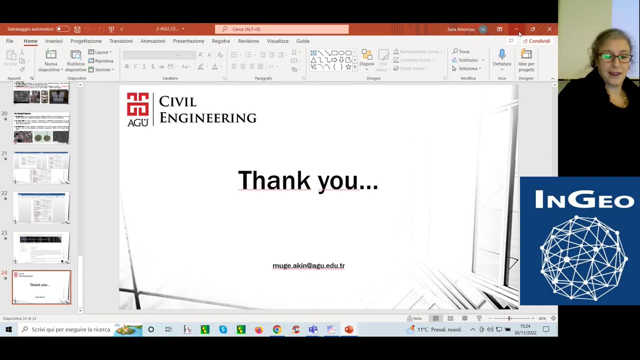 So thank you for listening me for university and for our department. So, if you wish, if you are ready, we can start with the liquefaction part. I don't know if it will work, or So my home or they can see the presentation. 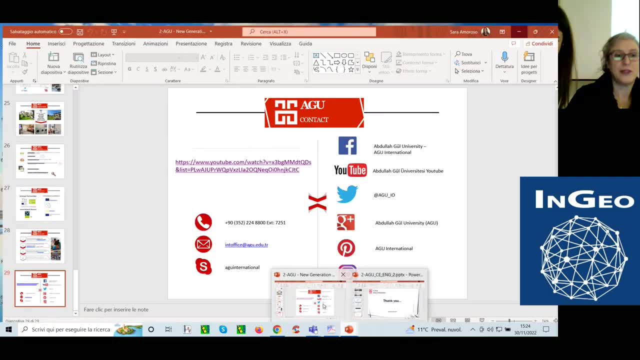 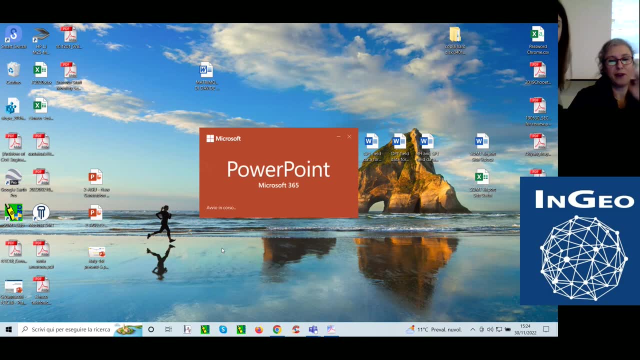 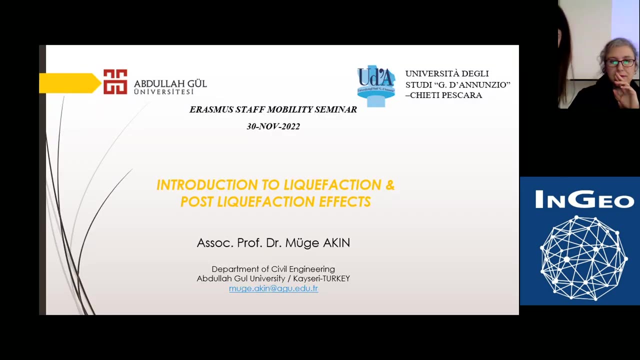 I don't know what happened with the connection with the screen, So the third one, so I can close this. I hope it's working If you want for this to put again the No, because I'm sure this is a function of that castle. 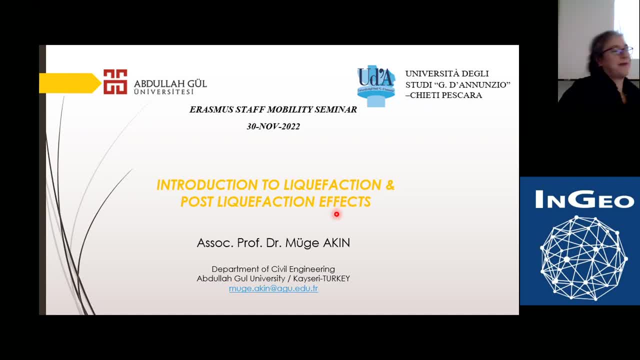 Okay So now I have the last. Yeah, you have the last set, So I like to give brief information about it. Okay So, I have a little bit of information about liquefaction. You have already learned- also teaching- about the liquefaction, but I would like to 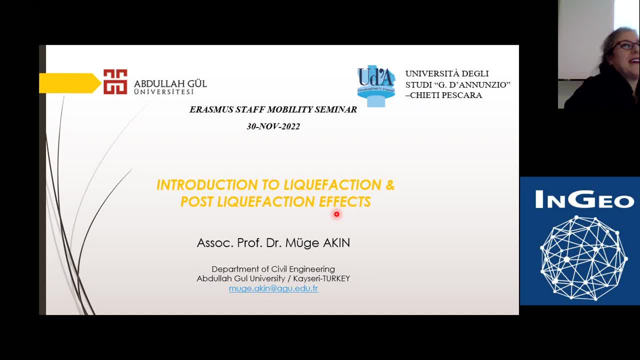 During that presentation? Maybe a very few: What exactly We've done so far And then what should we do. Maybe we can focus on that, or it will be having some questions in the end. I have some because we can find some projects or some. 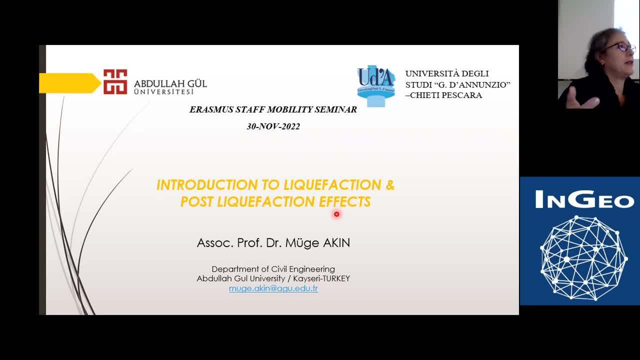 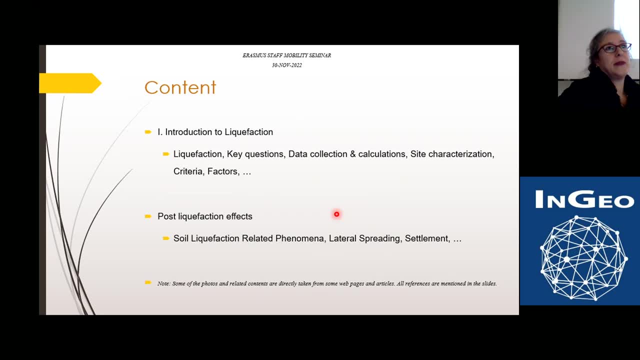 Things to establish. So I will give you some examples of some of the things that we have done During that period, because many things Were actually performed during that stage. So for today's part, I'm going to divide the presentation into two parts. 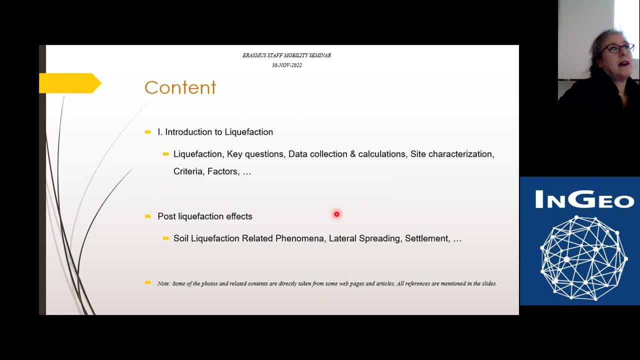 Firstly, I will Give some examples, some approach for the liquefaction part, And I will be talking about for the post liquefaction or secondary effects of the liquefaction after happens, Or what Do we need in exactly for the following projects. 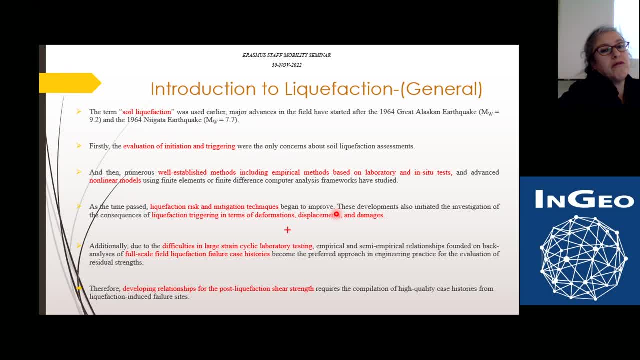 So, as You know, So like faction the term Is Used after, So Maybe earlier than that, They have Have an option to, Had to experiment. But after having this earthquake, With the fatalities, especially for the structural behavior of the soil, 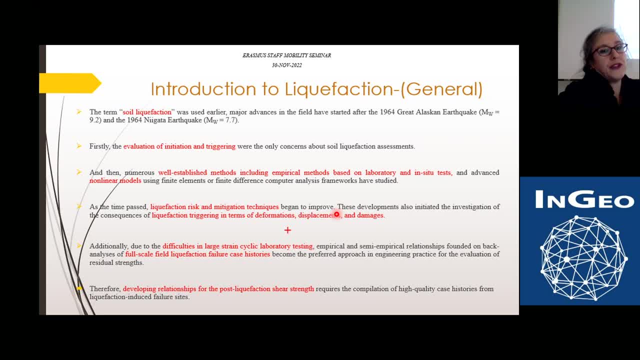 Behavior. It Comes To the literature. Let's say So. At the first Stage They evaluate And then they find the triggering mechanisms, Or Maybe baby steps Afterwards. Some methods were established, Like laboratory or institute test. 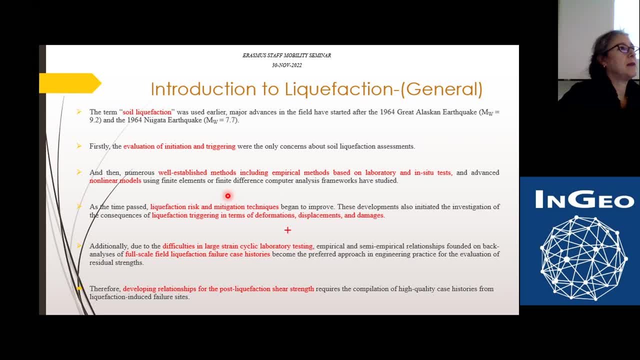 And some even non-linear models. They are using finite element Techniques or finite difference, And then It Comes out with the liquefaction risk And the mitigation techniques. So We have to consider the consequences of liquefaction triggering In terms of deformation. 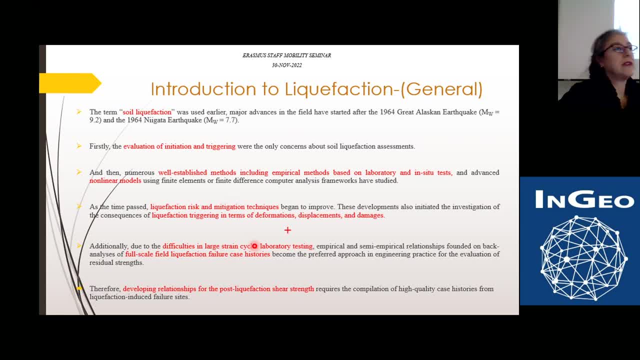 Displacements or damage. With an addition, There are some large cyclic Laboratory testing Approach In different countries, In Different places. They are all dealing with the liquefaction. As far as I can see, And Within that sense, 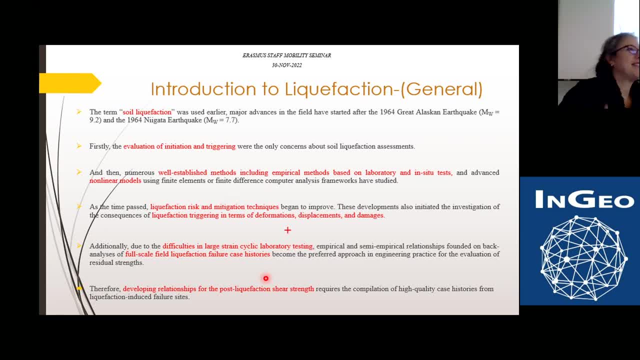 They are modeling Them With a full Scale And They are Modeling, And They are Modeling And They are Modeling Them Full Scale Afterwards. They are trying to develop Some Site. 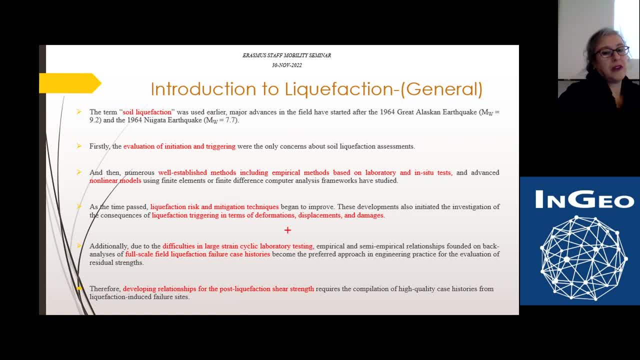 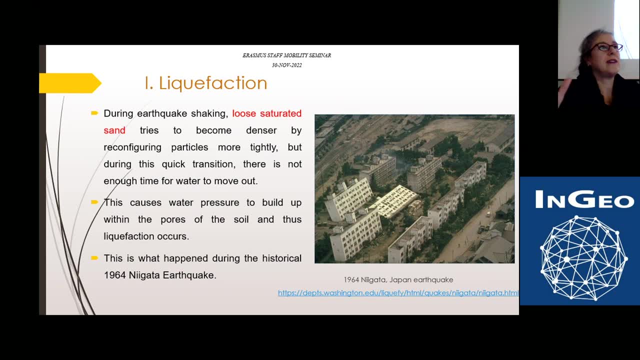 Specific Theories Or Empirical Formulas. This Is The Maybe General View. That's For The Introduction To Liquefaction. As We All Know, During This 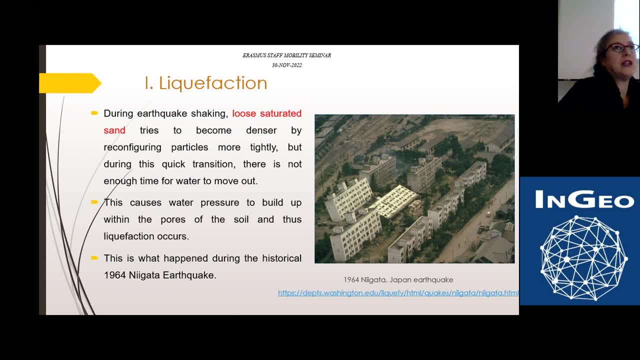 Time, So We Have Some New Updates. We Need To Also Discuss About It And What Else Within The Behavior. It's Getting Dancer Or Reconfiguring. 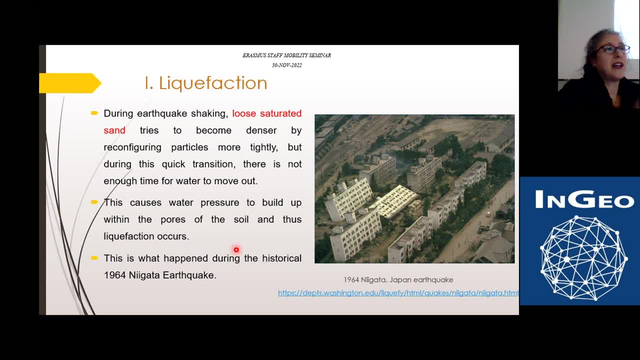 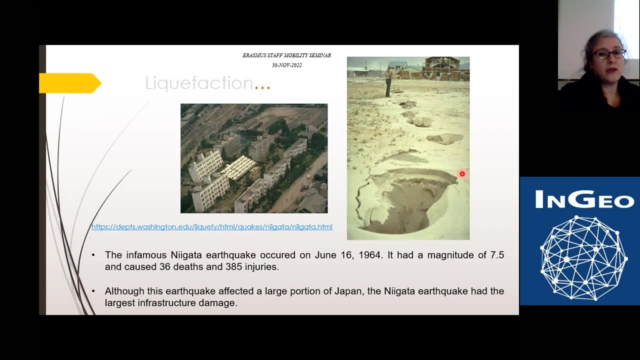 The Particles. So We Are Trying To All Solve The Mechanisms Or Model This Mechanisms. So This Is The Maybe Important Case For Us. 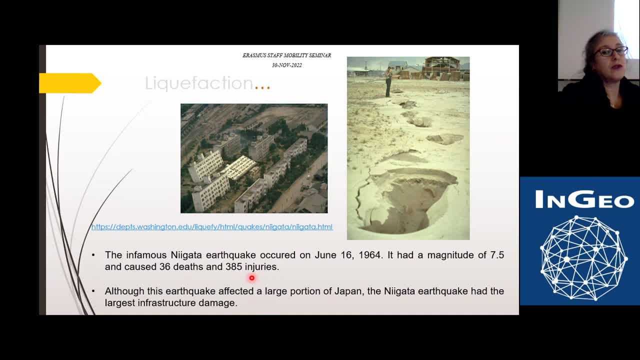 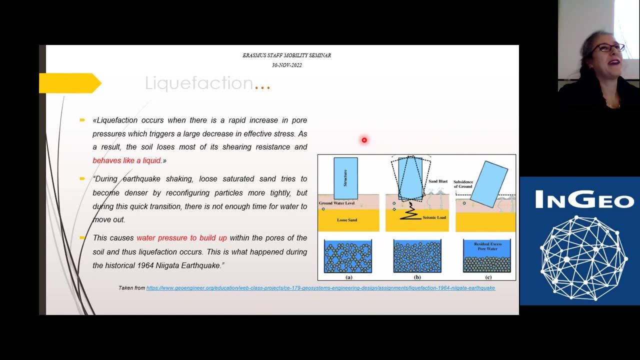 During The Historical Earthquake. So Here You Can See And Largest Infrastructure Behavior Damage That Occurred After This Event. So In General I Have Tried- 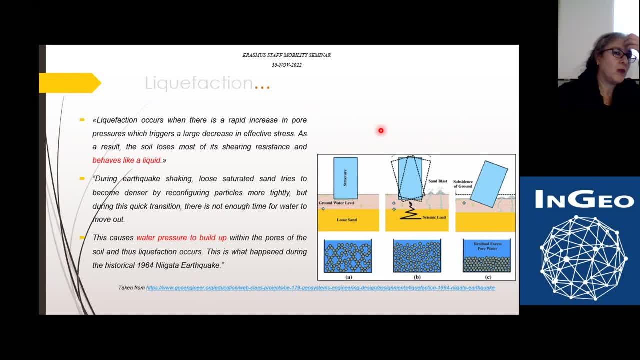 To Find A Way Or Definition For The Liquefaction. It's Really Hard To Understand What Happens In The Earthquake And What Happens Within. 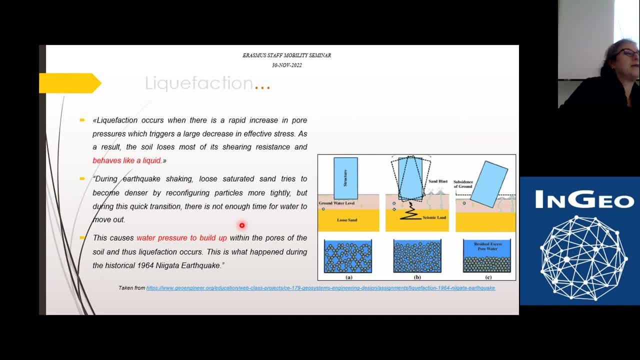 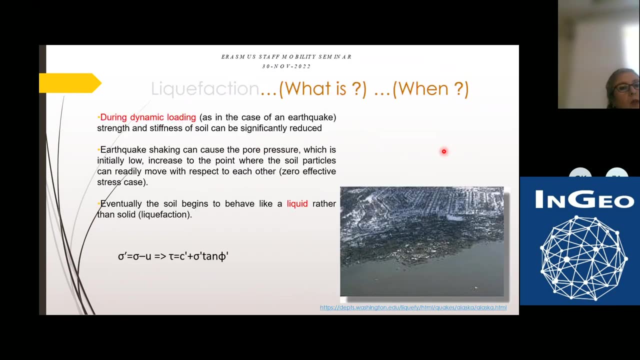 The Lose Material And Then What Else Within The Reconfiguration Of The Particles. There Will Be A Quick Behavior, Or When Does It Occur? 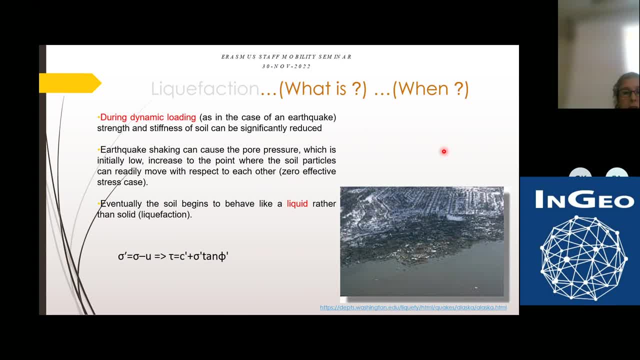 Depending On The Again Earthquake Shaking Can Cause The Per Pressure Level Change, You'll Be Having Increment. Especially, You Are Yes, And That Is. 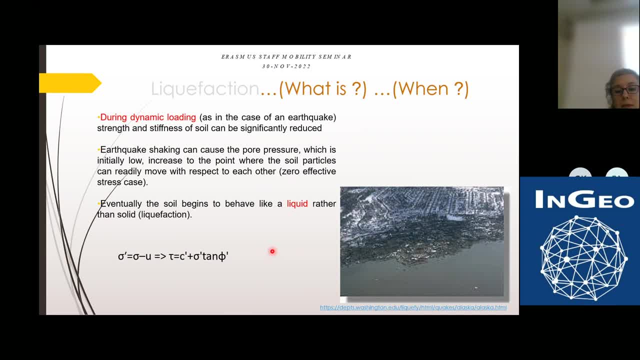 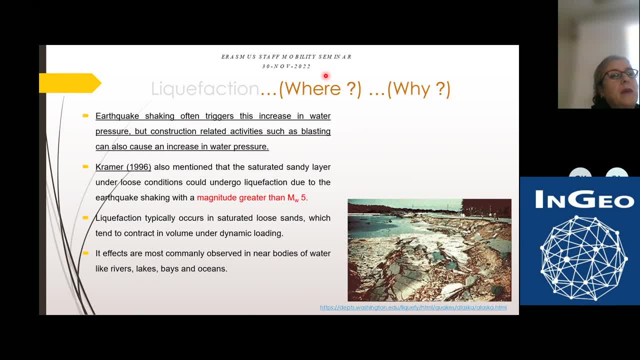 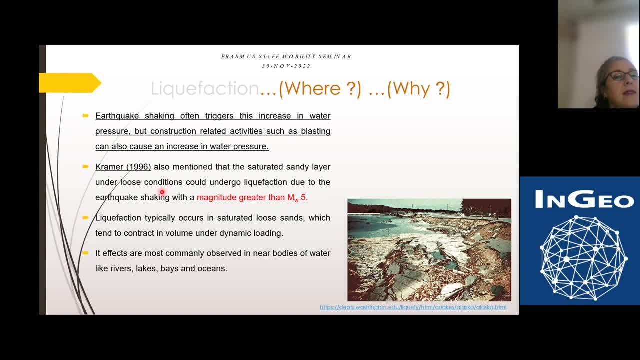 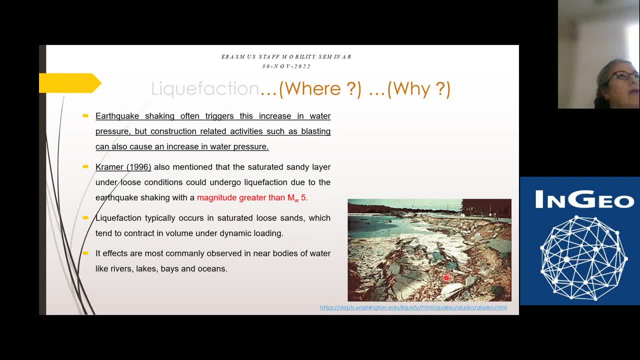 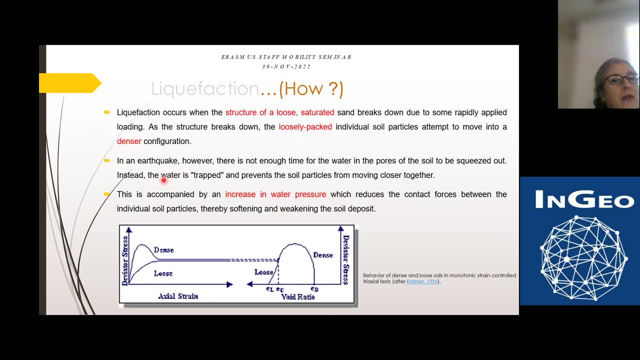 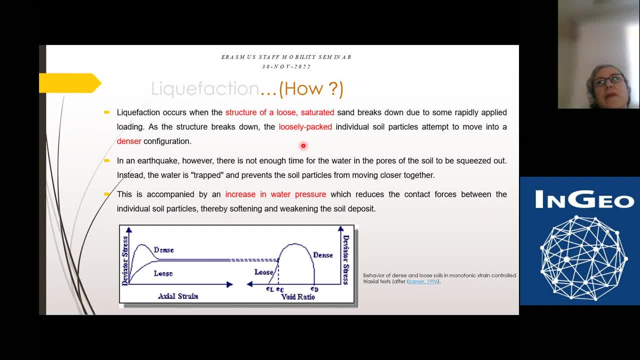 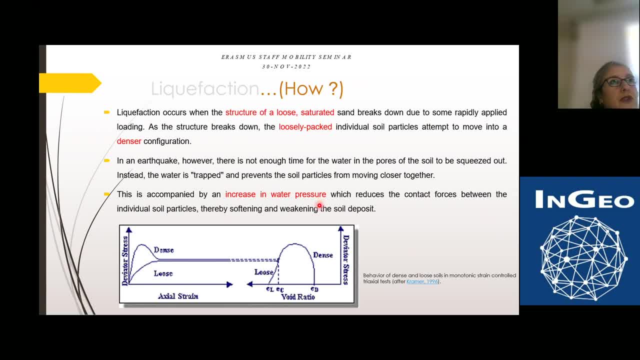 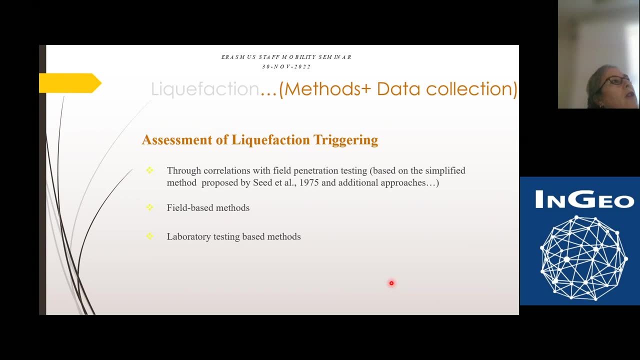 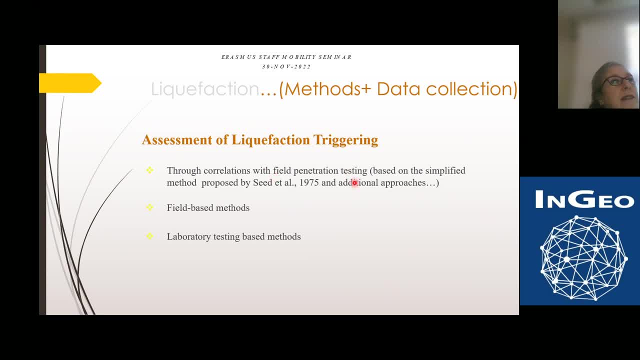 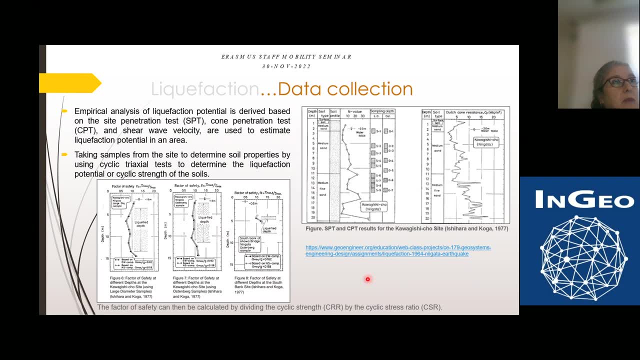 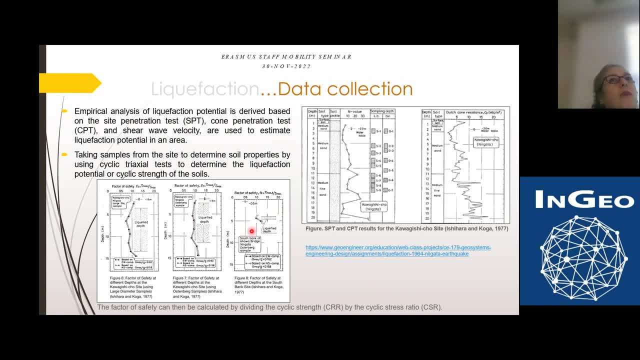 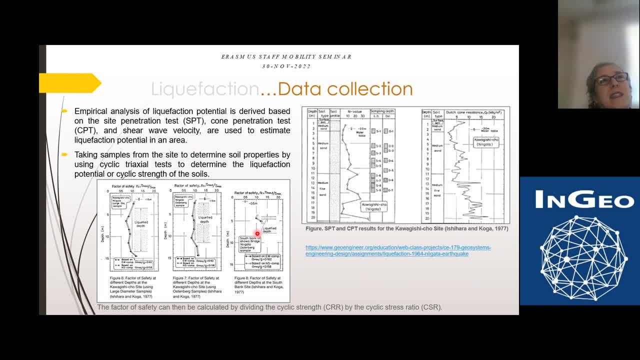 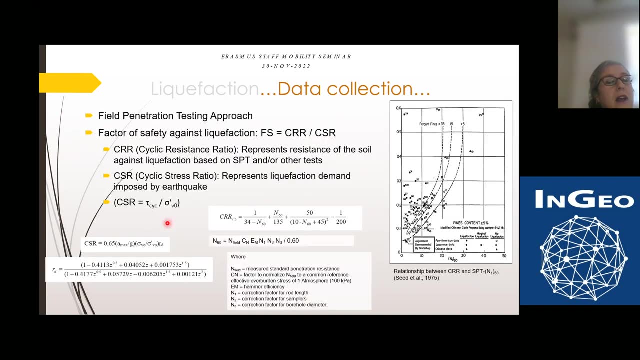 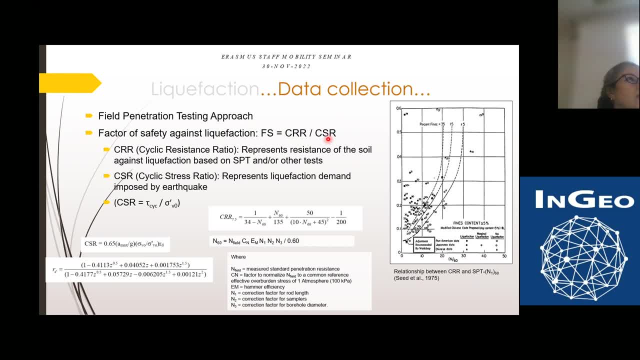 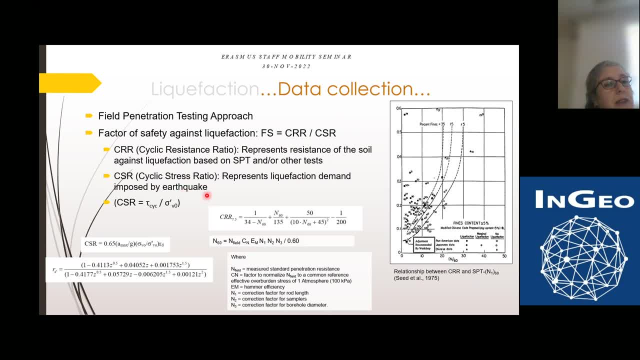 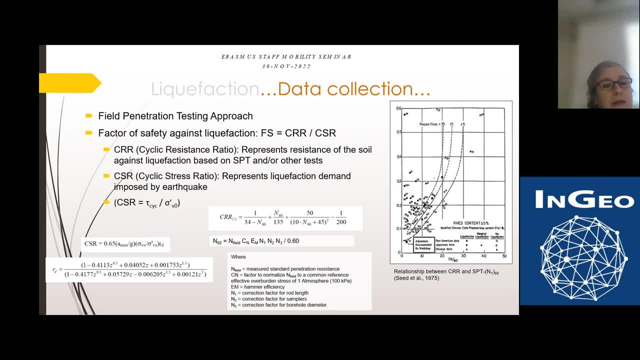 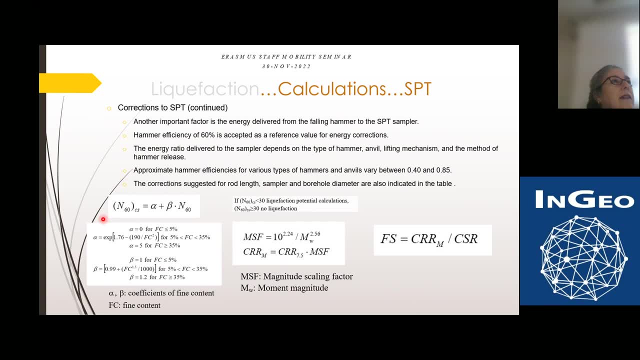 Of The Result, Of The Result, know, depending on that, when we correct and we had the factor of safety result, depending on magnitude, scaling factor, or even you are having some additional items or corrections that you need to consider for the fine content there are was a chinese criteria, as you all remember, but 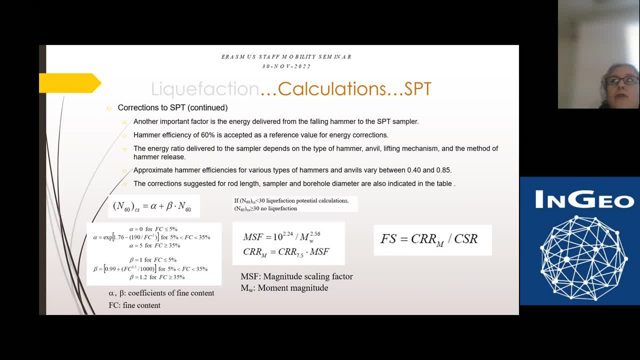 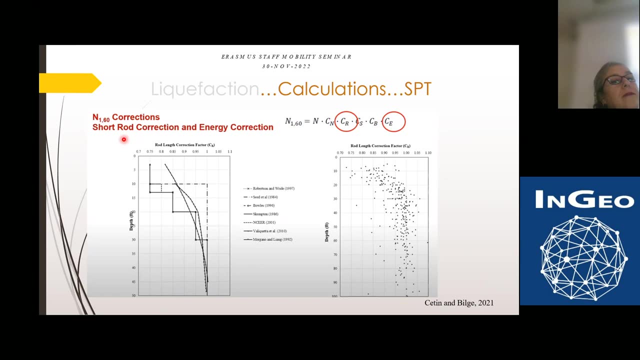 it is useless right now. so there are lots of updates. that depends on the fine content. even so, as far as i can have the talk from chitin and bilge just recently, they are assuming that the road connection that we are having, for instance for cr it looks like, should be updated. we are 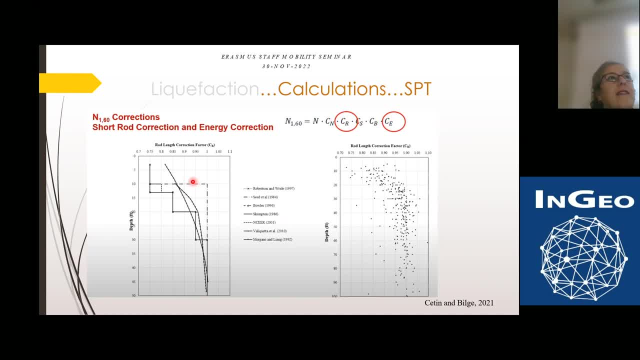 considering that we are taking the road and then having the application for the correction, or they are also thinking that uh energy ratio of the uh spt. so there are some unknowns and still we need to find out. for the corrections are for the applications of the. 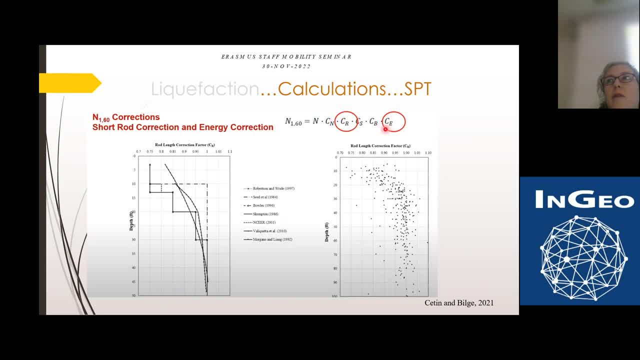 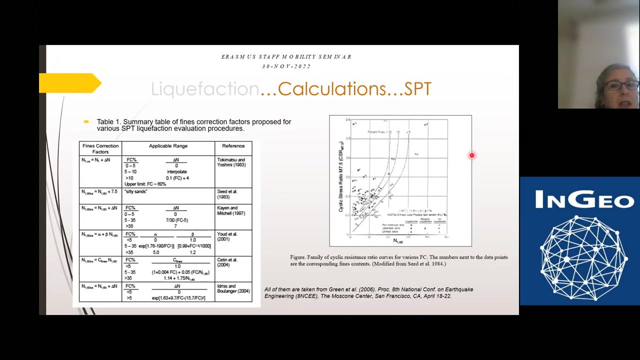 formula because, uh, in italy, how many percentages of energy ratio you are using for spt, is it? yeah, okay, okay, but there are some actually apparatus in order to measure the energy correction, so it is necessary to apply maybe in instead of having this item, so spt again. you can find many correction factors with the fine content. there will be some applicable. 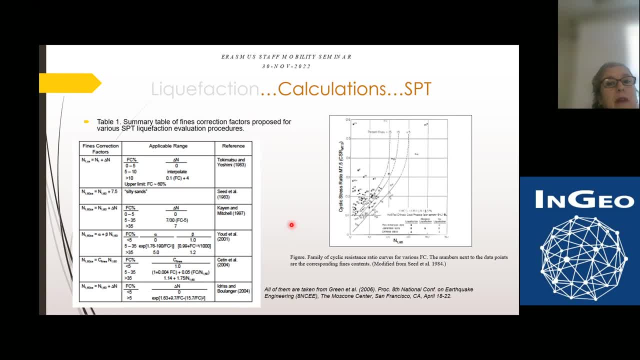 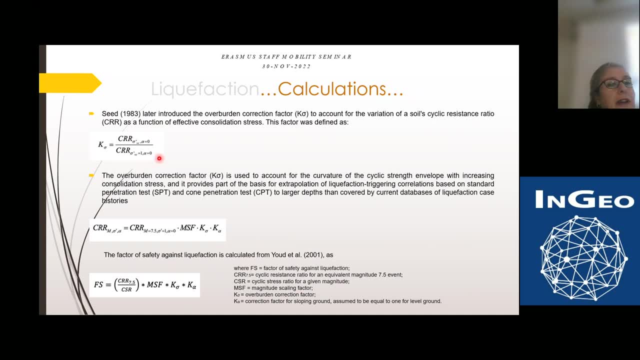 range at different again procedures and some empirical formulas. and it continues why? because we have overburden correction factor. even you can add some sloping around correction factor. so if it is a sloping area so you have to consider additional correction. it looks like getting uh complicated with the spt based or even cpt based. 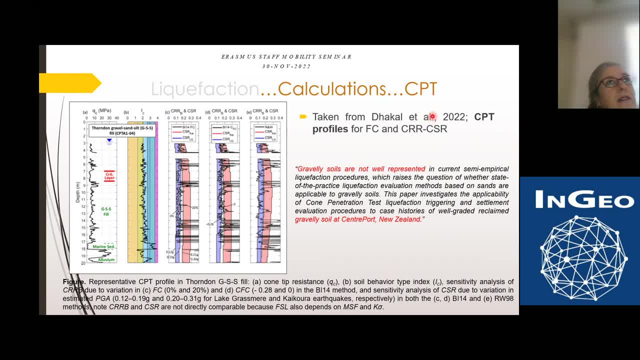 i have just taken recently as a cpt study. you are all familiar with the concentration testing they have performed within the critical layer which is related with the gravel soils. so here you can: comes to our mind that gravel soils you have and you are dealing with the some cpt applications in. 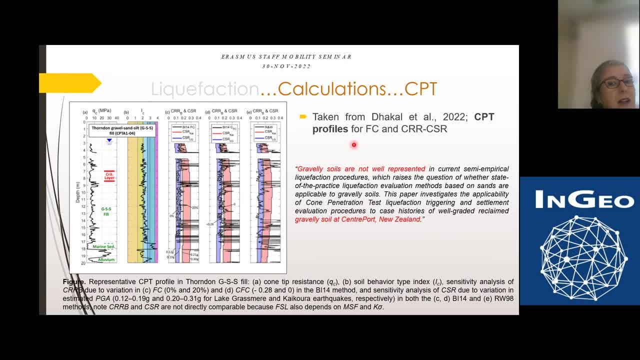 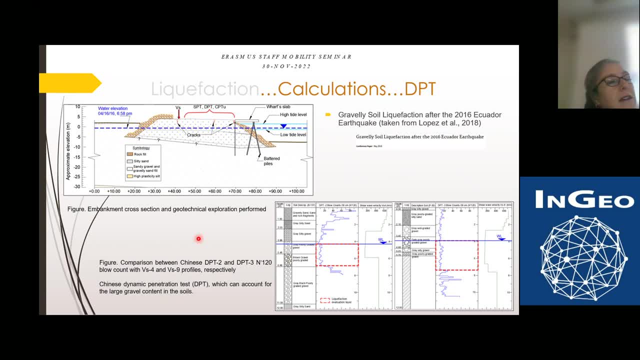 order to get the liquefaction analysis or etc. it's a kind of approach from new zealand and i have also come across dpt for the ecuador. i don't know how you're familiar with. it is called chinese dynamic penetration test. they have also compared with, again in gravel soil in. 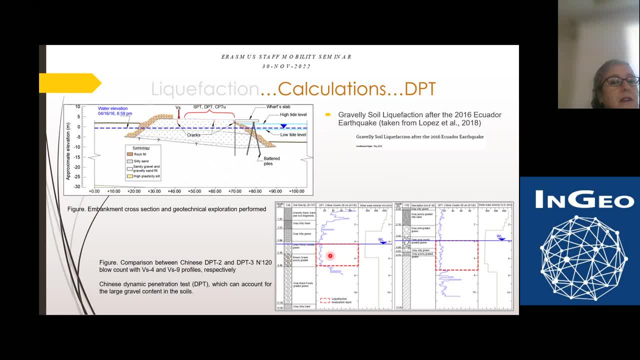 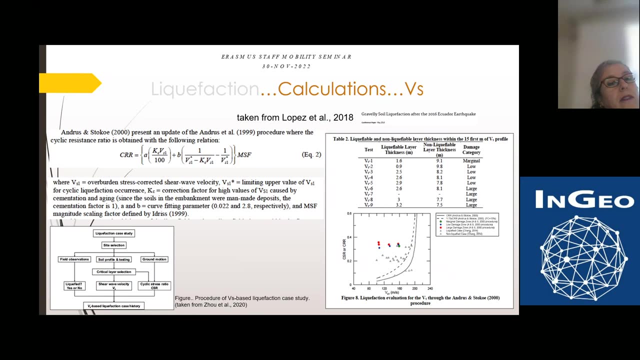 order to get some results for the likable layer for the critical area. so there are still ongoing projects and new, maybe updates for the applications and when we come through the shear wave velocity approach there are some one, especially the famous one- you know anderson's talk that we are using it a lot, but there are some again gaps or some new updates. 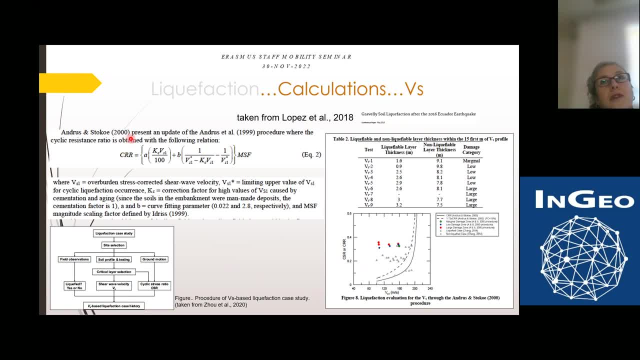 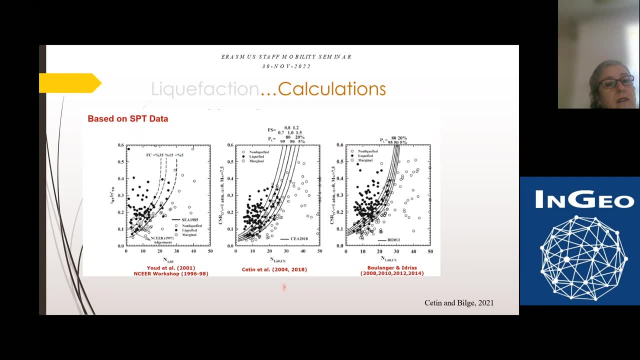 that i have to mention that i am going to show some figures and some recent references and, within the returning spt data you can have from different areas, when you have a look with the different states and with different years, you are actually and we are actually having more data. 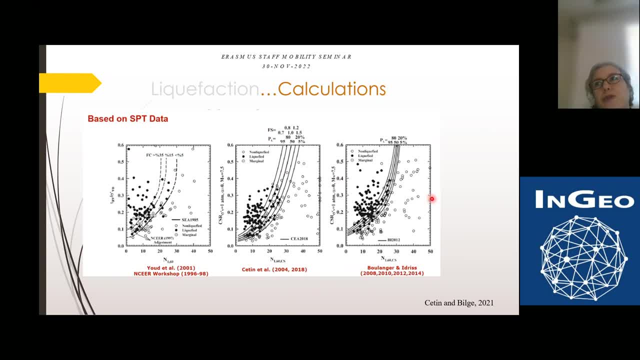 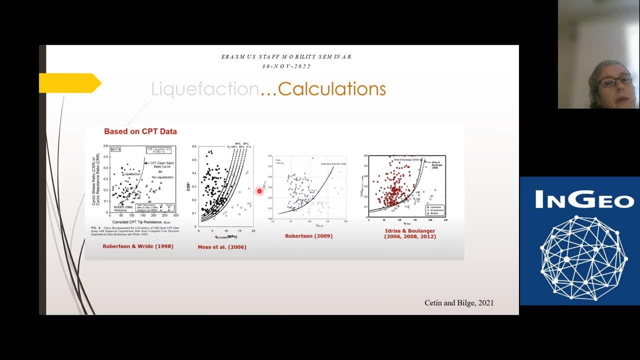 that means that you can be in the safe side and you can be sure in order to study. but how about cpt, for instance? again, it is valid. you can have different approach. within the address and bulange, for instance, they are increasing the database again and then having different curves in order to be sure which would be the liquefied and non-liquified. 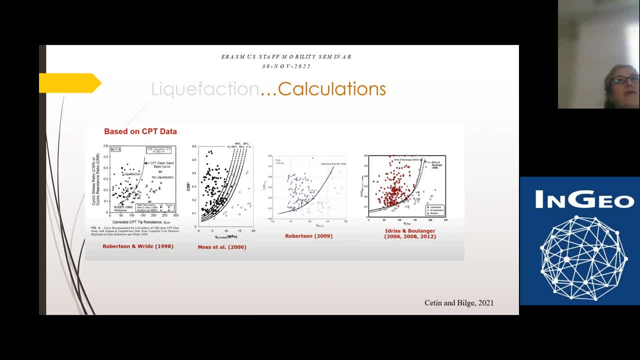 but in somehow there are some researchers even could not update themselves or couldn't use the recent version of the methodologies. even they are maybe losing themselves inside the research or other things. so this another critical issue: we need to clarify all of the items and for the vs. 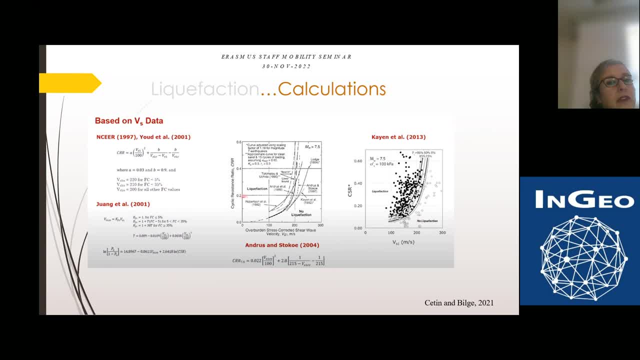 calculations. as i mentioned, we have understock. it's very famous and there is a new study which study with Cayenne, which is also related with the shear wave velocity, depending on the different cases. So if you have the data, you can even try or you can compare with SPT. 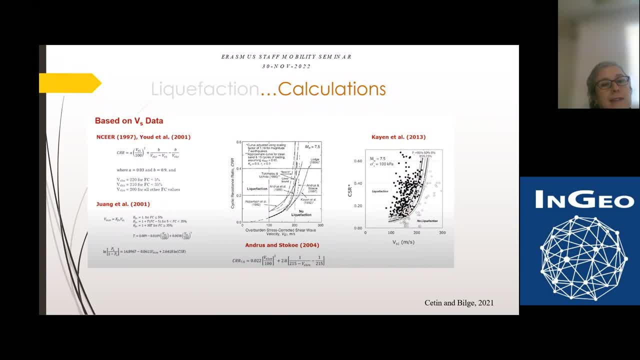 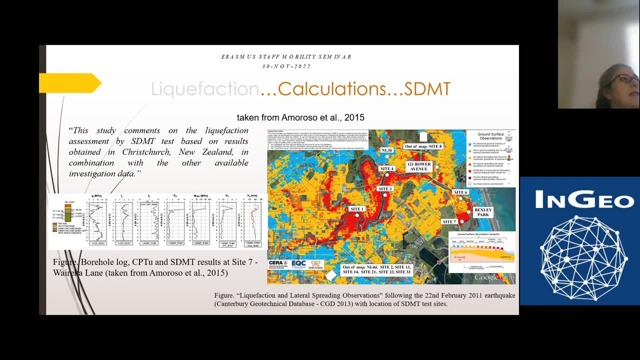 VS or CPT etc. But when I arrived and we talked a lot with Professor Amarosa about SDMT, there are some still works ongoing at that stage and it is really worth it to work on it. It's also there will be some comparison in between the CPT and SDMT And she showed 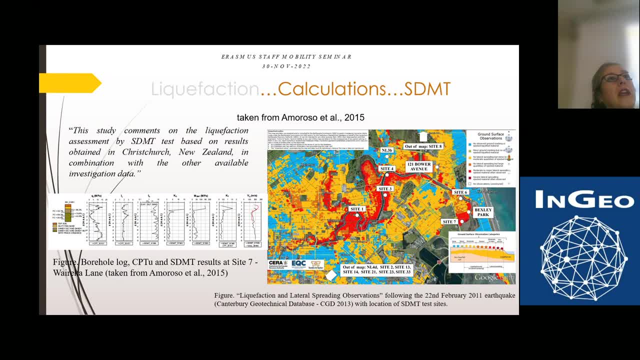 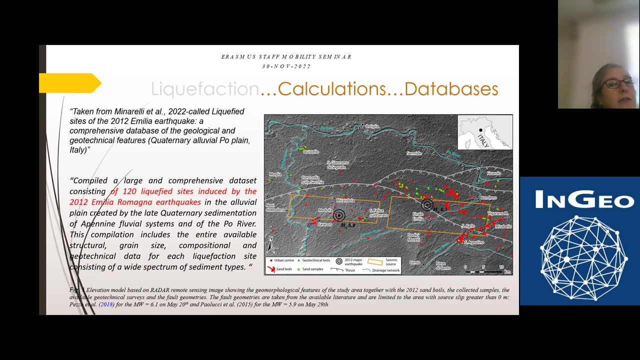 me and shared with me some of the important items. This is also important and critical thing for the liquefaction behavior and for obtaining and updating the cases. maybe I should say These are the calculations part, But how about databases, For instance? I would 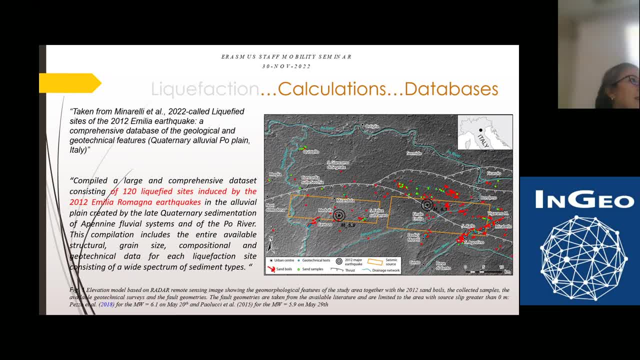 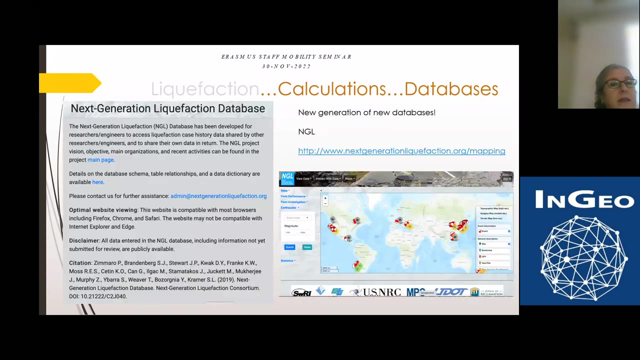 like to share a database from Italy. They have 100.. 120 cases or even some special cases that they are collecting as a sand boil or some lateral spreading or liquefaction behavior. But when we think about the worldwide stage, that means that you need to also criticize the effect of the database that we are having Nowadays. maybe you 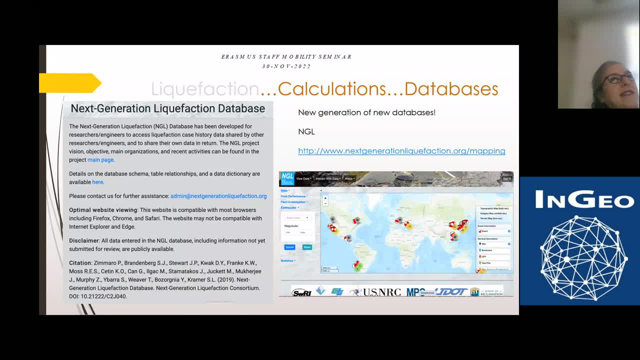 heard that, like attenuation models, like the new generation attenuation models, that's also a new generation of new database, And that's also a new generation of new database And that's also a new generation of new bases, depending on next generation liquefaction database. I have searched a lot, But there are still some missing data that you need to also update for all over the world And in some sense, the data expansion depends on the quality of the data. another issue that you need to consider: there actually a group of purpose grammar that also involves in and 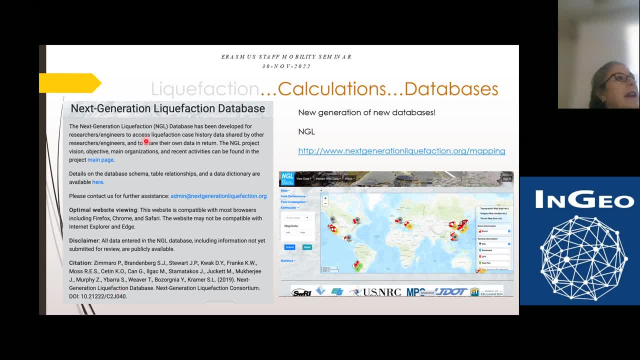 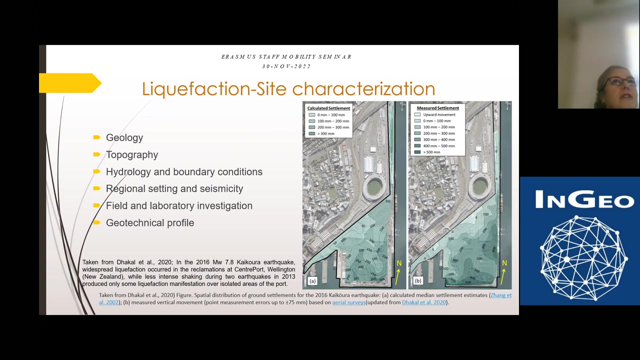 Generally having some meetings depending on this NGL database. Maybe there should be some additional references we need to add and we need to talk about it. So until that stage we have already calculated, We had the database, and what happens or what if we have the different parameters, like geology, topography or some hydrological conditions or what else, some regional setting? 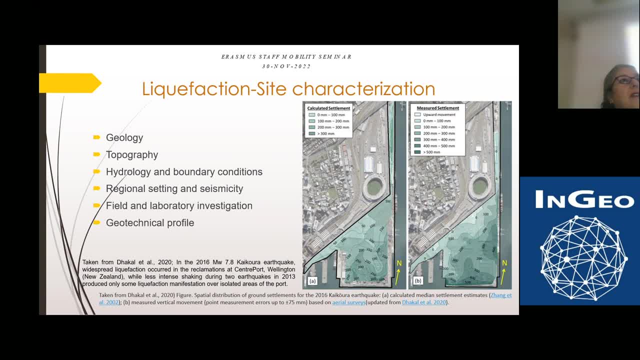 So the seismicity would be critical for us- and some field and laboratory investigation- they should fit pretty well- and some geotechnical profile. And here you can see a very recent data. They have calculated the settlement in that region but they have measured different settlement depending on liquefaction base. 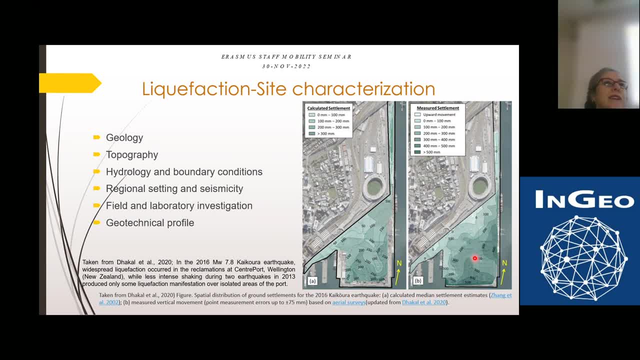 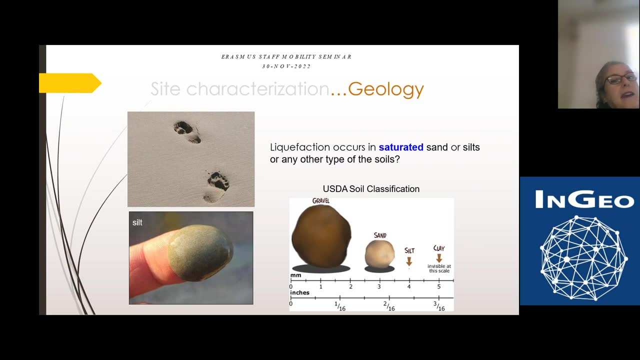 So that means that you are calculating, but you have to also confirm that if it works at the field or not, We have to be sure. That's another item that I need to mention. What else for the geology when we return to our case? 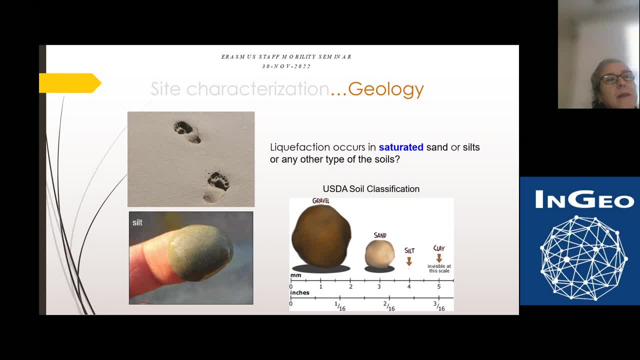 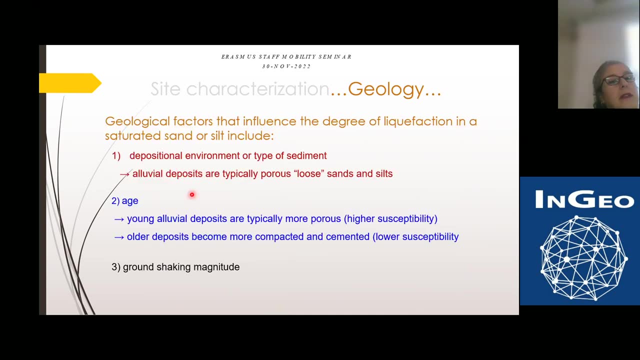 Yeah, we are all knowing that sand or some silt, but how about clay material or gravel material? There are still some unknowns and there are still works ongoing. at that stage With the factors, we need to also consider the positional environment. 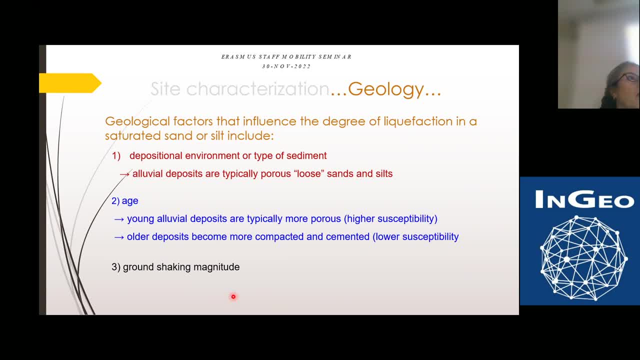 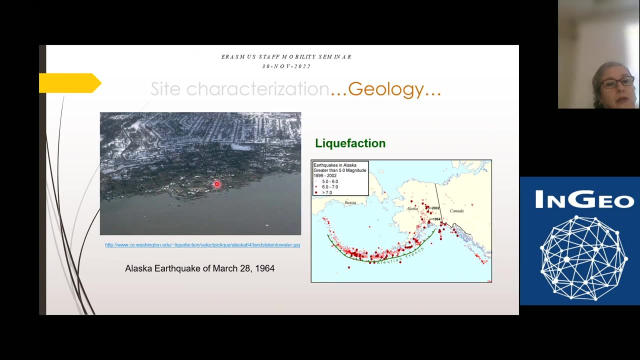 Or even air, Or the size of the soil, Or the age or the magnitude. So we have to divide or maybe we have to look for some special parameters in order to connect the database. So here you can see the effect of the geology or related with the behavior that it may occur after a liquefaction or even in these areas. 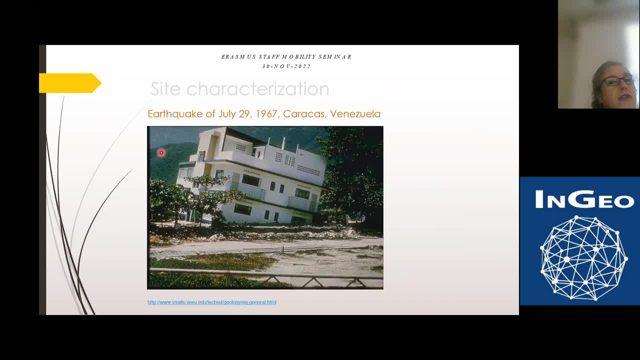 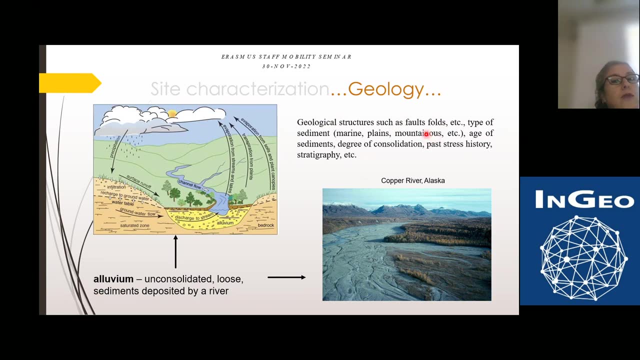 Or you can see the structural behavior, but the foundation because of the liquefaction that may occur after a liquefaction That may cause the problem for your case. So for the geology, especially geological structures And faults, Both types of sediments. 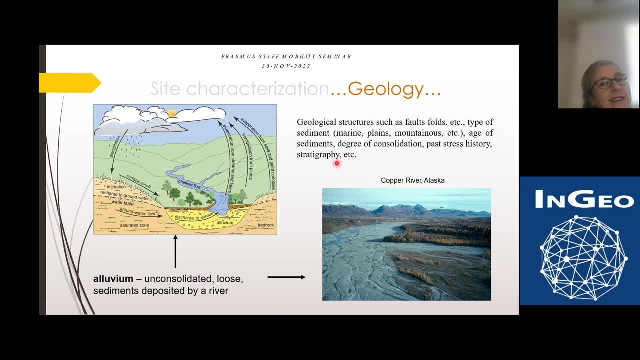 We have to also go deep inside the area, because age of sediments would be also critical for us. I don't know how size or I mean the scale effect would be effected. We need to have a local size, local scale or we need to make it bigger size. so we have to be sure again. and, of course, degree. 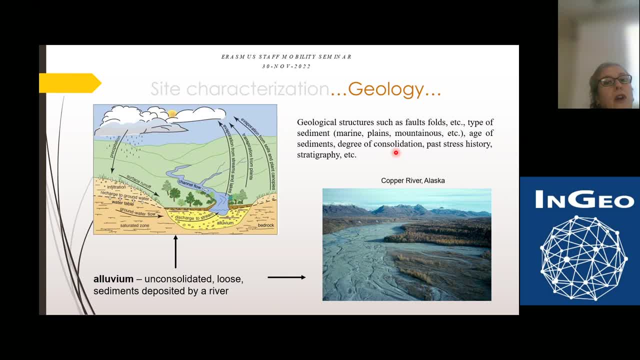 of consolation, depending on the clay material you have or past stress history, how we can measure or how we can understand that. so we need to have some geotechnical profile or site investigation models in general and, of course, 3d one right now. so, as you can see some olive oil material here, you can 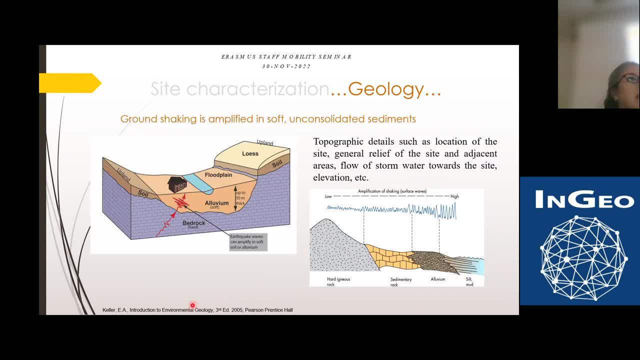 have, and what else? amplification. so do we need to consider both amplification and liquefaction at the same time? yeah, maybe, but we should also work and then think about it, because it's also related with the topographic activity. we should also consider that i would like to emphasize. besides, there are 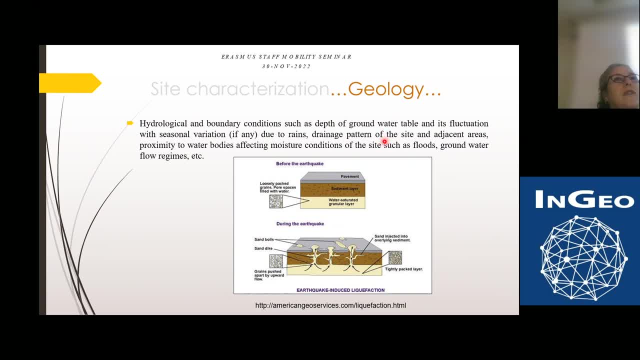 some hydrological conditions. so how we can measure the depth of the groundwater table or how can we be sure that the depth is exact depth for us for our analysis. we are assuming some kind of behavior that occurs in the actually soil type, so it depends the rains or drainage pattern. 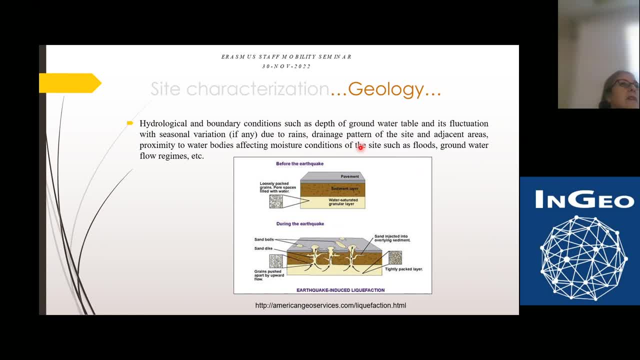 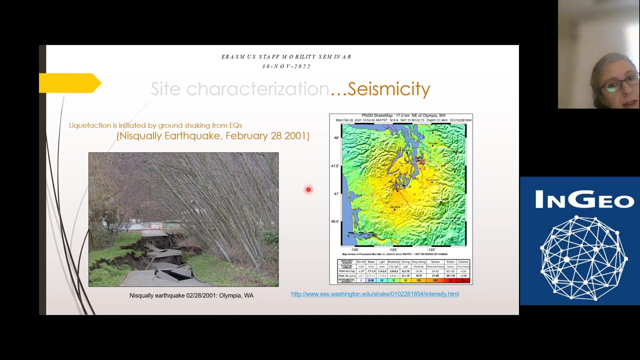 etc. so you need to have an old model, including maybe interdisciplinary approach and when we consider the effect, especially in the moisture conditions like flooding or groundwater, you will be facing maybe liquefaction behavior that may occur just frequently. i have a study that i would like to emphasize that occurred in washington state with a very low seismic activity. 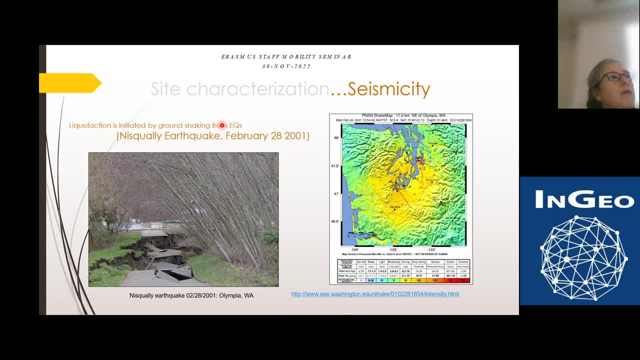 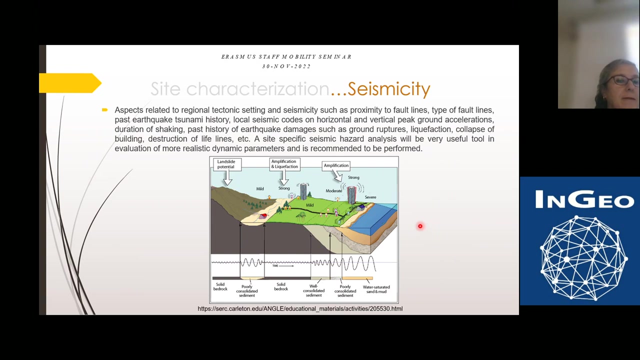 but there are lots of actually liquefaction behavior observed within this range. so we have to look at the different fields in each region and realize how significant the magnitude or which magnitude levels that we can have, which amount of accumulation or liquefaction that we can have and others may be. point that i have to be, i mean give information or a value. 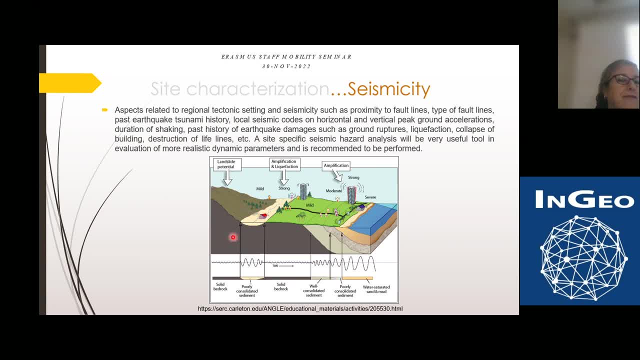 so for the seismicity, again we have some potential. it's a nice actually figure including all of the items, but we need to also deal with the we are having, how we can be sure that there will be a boundary in between the layer or depending on the fault activity or some past earthquake or tsunami history or etc. so there would be a kind 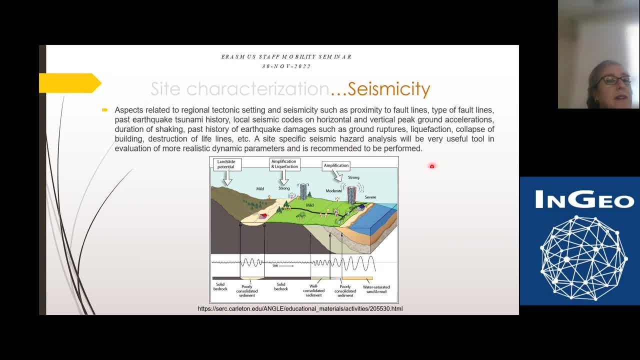 of site-specific seismic hazard analysis should be done for the relation of the parameters and the performance. sorry, i hope i don't get bored you, but yeah, it's the long topic. so if we call or find the parameters, but i can add additional ones like the factors. 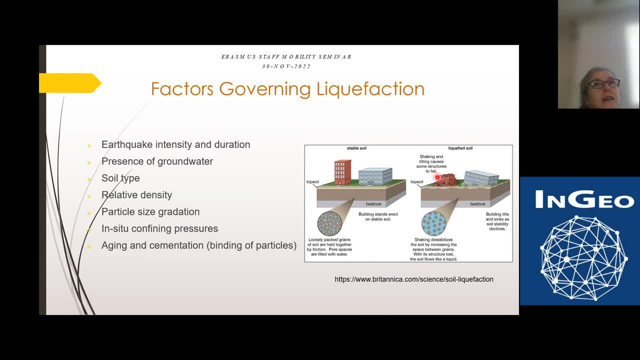 can i add instead of magnitude like intensity or duration of the earthquake? yeah, there might be possibilities. so it also affects the liquefaction behavior. again, it's related with the groundwater and the other things also similar. but besides we should also have institute confining pressure that occurs around the material. 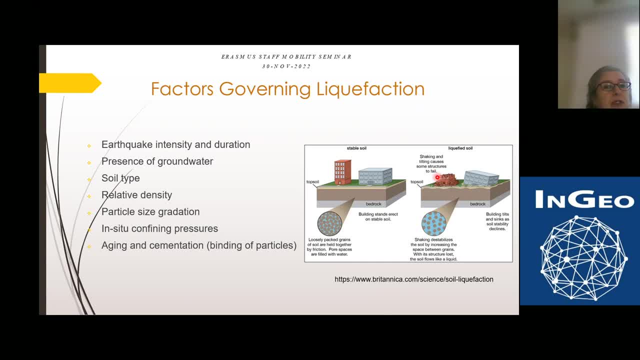 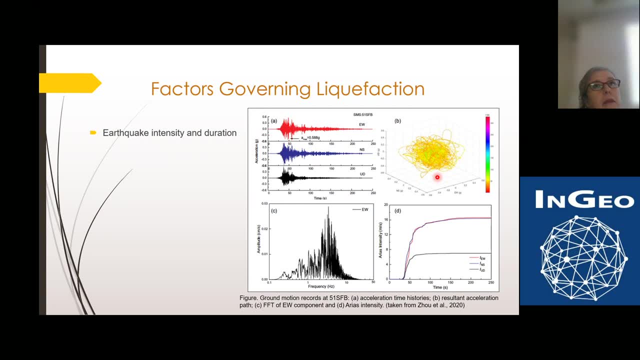 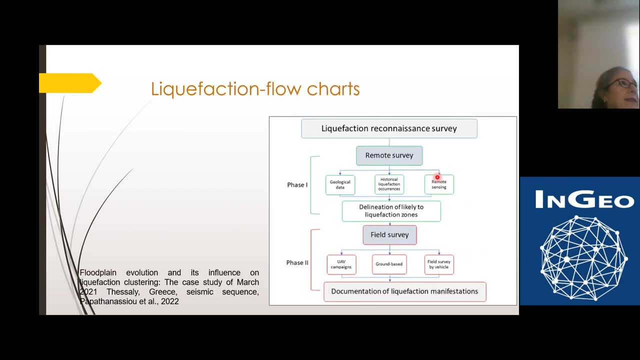 and these are the maybe we should consider especially intensity and duration. we have to make somehow correlations in between that, maybe, or like the presence of water that i am repeating. so how we can do that, i search some of the approach. there are some flowcharts, okay, you. 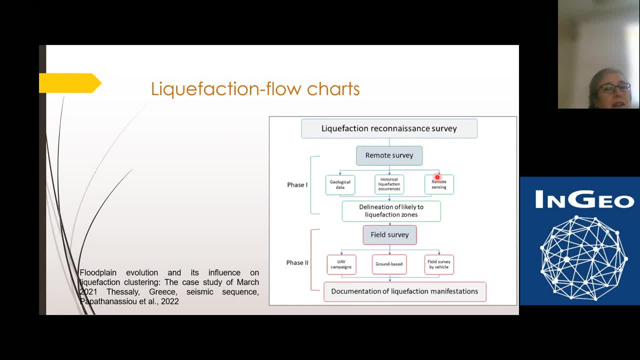 can take one of it, for instance. it's a very recent one and they have two phases, for instance, and with this they have the data they are collecting with the survey and then having field survey and then some finding for liquefaction manifestations in the area. it's really hard how we 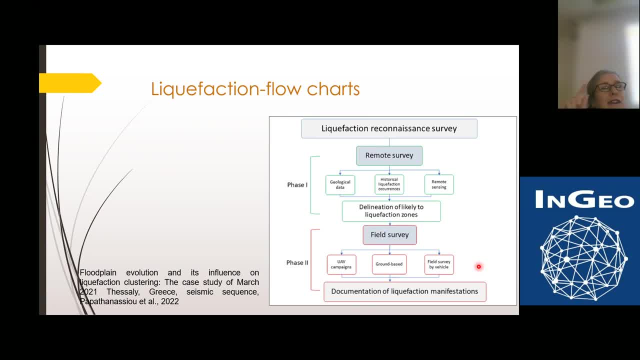 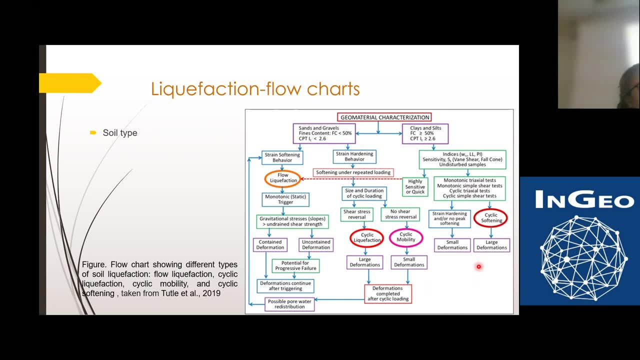 can behave for a flow chart, or do we need to have our for each country or for each area? we should be sure. and what else? this is another flow chart. for instance, you have the soil type and here you can see, with the differences and the behavior of flow, liquefaction or some cyclic mobility or softening. 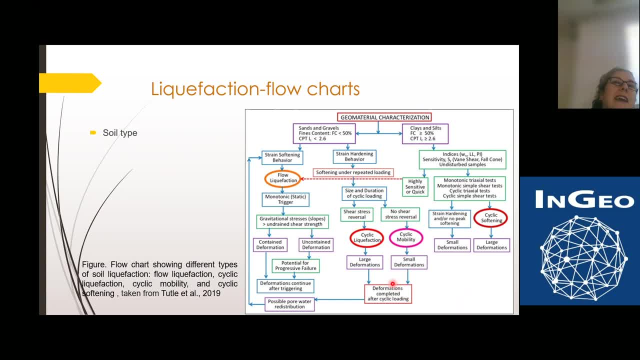 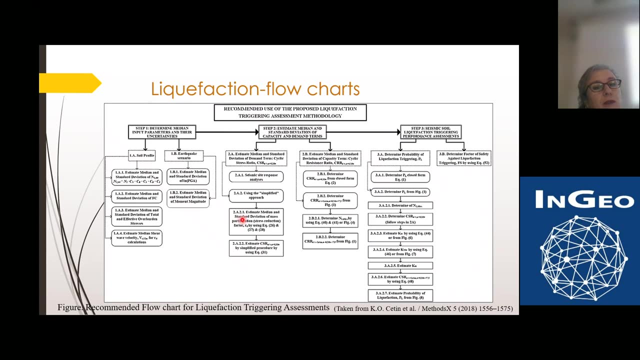 behavior, which case or which point should i use and then complete the behavior for all general liquefaction approach. this is another item that i have to also give this to you. i found another flow chart which is related with the liquefaction triggering assessment. so how i can assess or how i can define the liquefaction, the 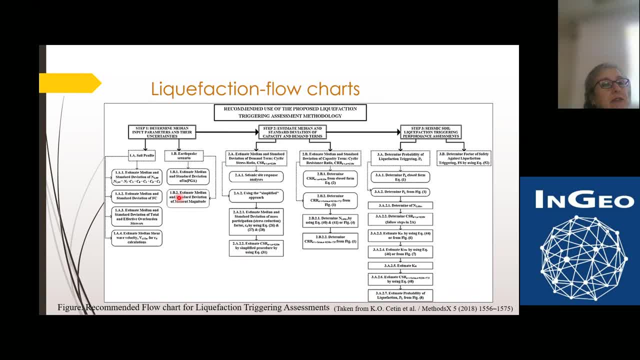 liquefaction or how i can define the liquefaction or how i can define the liquefaction. on the methods, actually you can have the different soil profile- i don't know how it clear, but it's the recent work of again chatting at all- and you can have different steps by including: 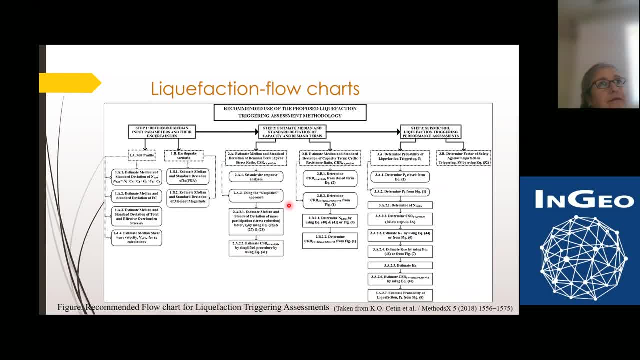 like the even such response analysis in the system. so which flow chart should i use or which methodology should i take? so this another question. so until that stage i have tried to figure out and give some questions, or just brainstorming for the liquefaction part. if you are not get bored, i'm going to continue with the 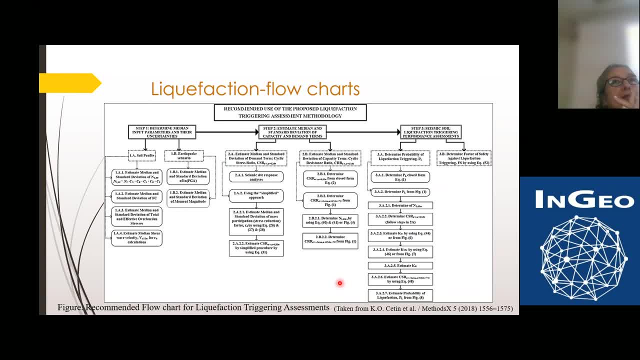 post liquefaction part or, if you don't have any questions, no, it is fine. sorry, my voice is getting maybe sometimes stable because of talking. yeah, yeah, actually i heard from their approach, especially depending on the methodology that they are having working on, probably, yeah, so we need to be updated all the time, and then it's really hard while you're doing your work. 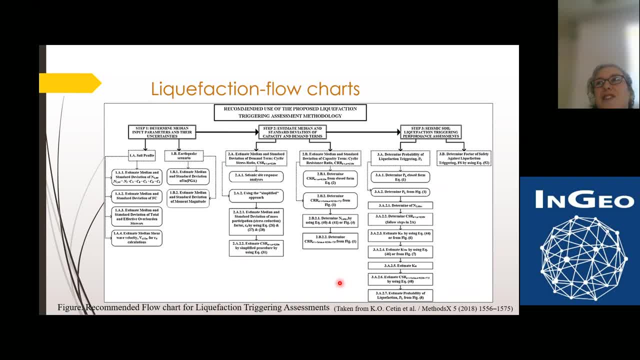 and then you need to update all the time and then it's really hard while you're doing your work and then you need to, Yeah, especially for the road length also. it's also, yeah, critical. Short length is like one meter or less than one meter. 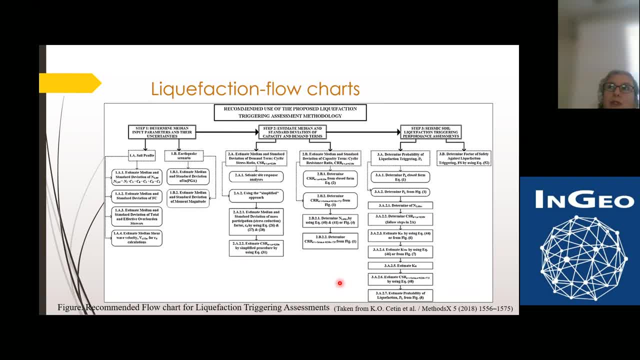 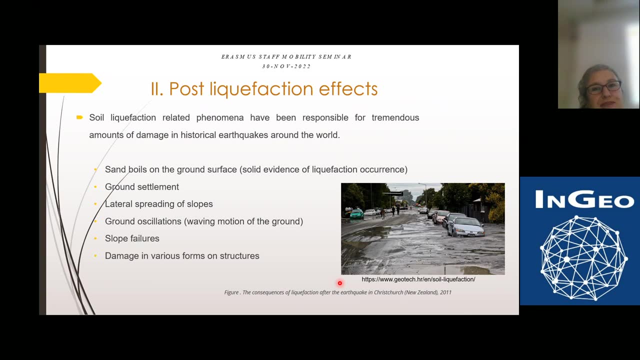 Less than, or it depends. How can we be sure the firms are applying the exact amount of the road, or are they giving the exact length of the road? Yeah, So I'm going to continue with the post liquefaction effects. In here you will see some secondary, maybe- moments that occurs after liquefaction, such as, as you know, sand boilings. 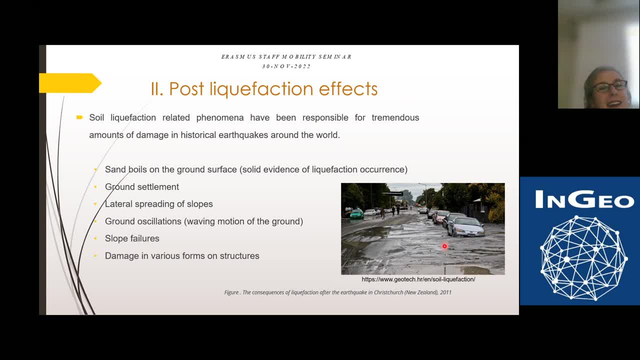 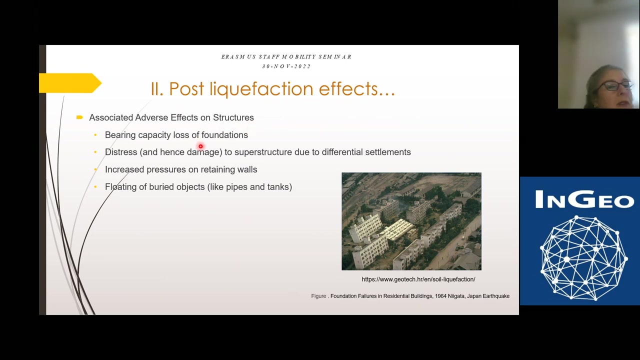 It's a very nice case for us- And there are some settlements, some lateral spritzings and some ground oscillations, some slope failures that may occur And what else, Some damage in the various structures. So, besides that, we can have some effects on the structures, like the bearing capacity loss that we can have. 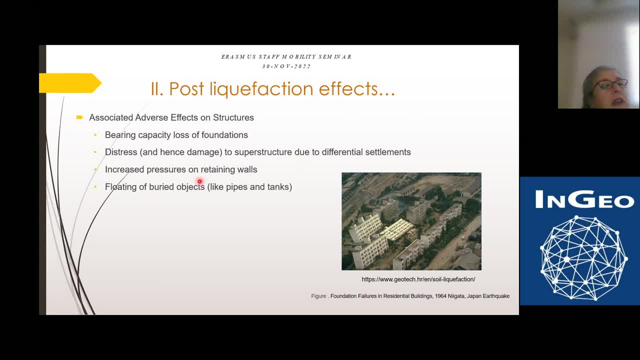 or some differential settlements, or some increments in the pressure of the retaining walls, or some buried objects like floating inside, especially the pipelines. Maybe the main problem that we can have? Yeah, Because of the liquefaction failure- And I would like to share this- foundation failures. 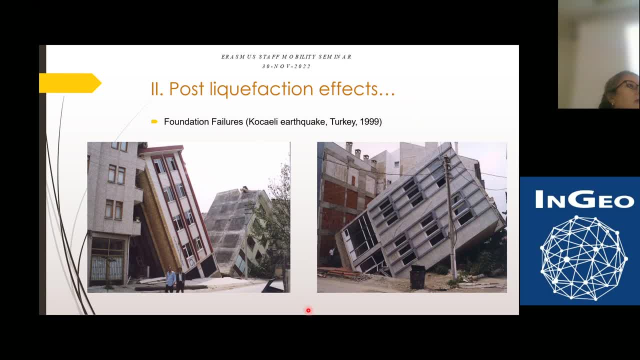 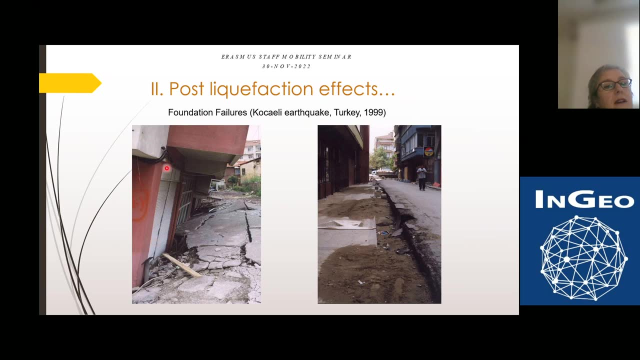 They're all really famous after 1999 Kocaeli earthquake. As you can see, the structures are seems OK, depending on that stage, But the liquefaction behavior, or even in here, as you can see, with a settlement of 35 centimeters or maybe more than that. 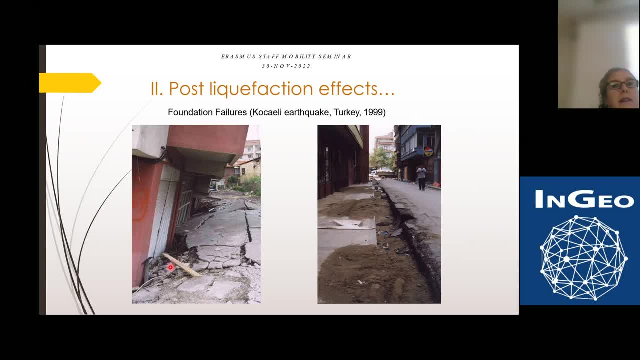 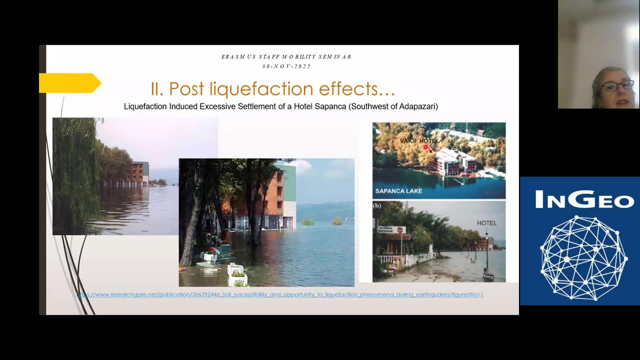 they have had this problem: 1999 earthquake or with this, as you can see. So these are the foundation failures. What else You can have? liquefaction induced settlement and, of course, lateral spritzings. So, as you can see, the hotel moves towards to the lake because of the lateral spritzings behavior. 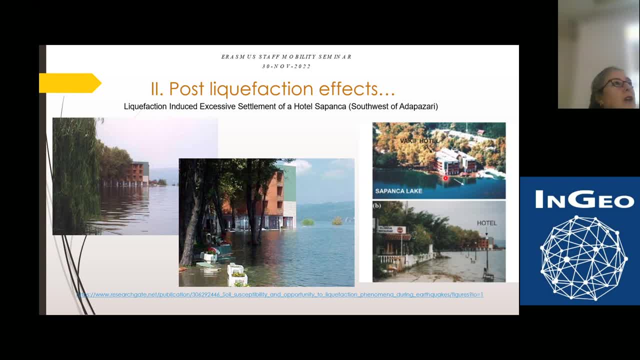 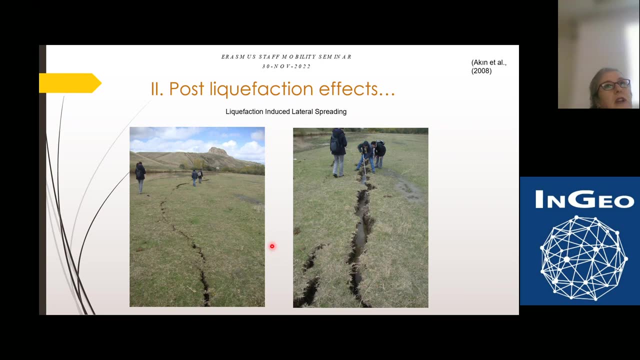 It's a huge and important case for Are even in geotechnical history. Maybe I should say that there are some approach for it And what else. There are some lateral spritzings that you can observe, especially near the river, And then you need to also measure, and then you need to go after the earthquake in order to get the data. 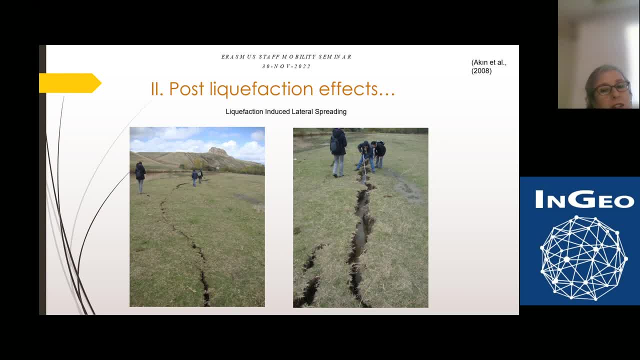 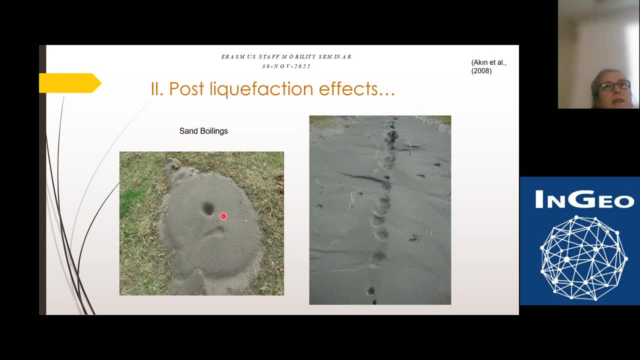 But it's another thing that we need to consider Additionally: sand boilings. How Would be the amount of the sand boiling? So what would be the radius that you are having or the material that comes out? Also, we should add the kept soil behavior. 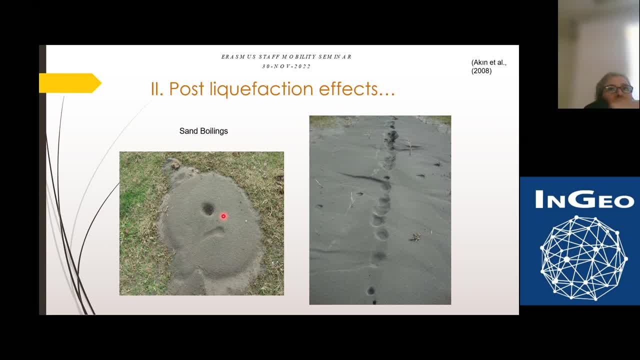 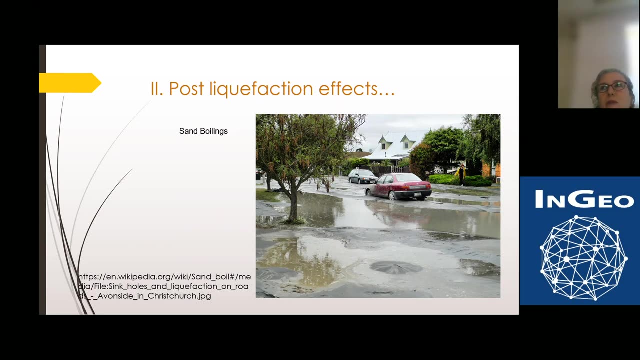 You can have, maybe unknown material that does not allow to. material goes up, So we have to also study on that. And with the sand boiling, you know, Christchurch is the typical one And Professor Amoroso is Really worked there, as far as I can see, collecting and making lots of experiments. 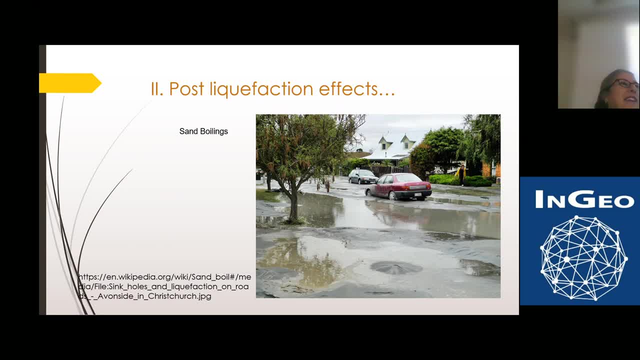 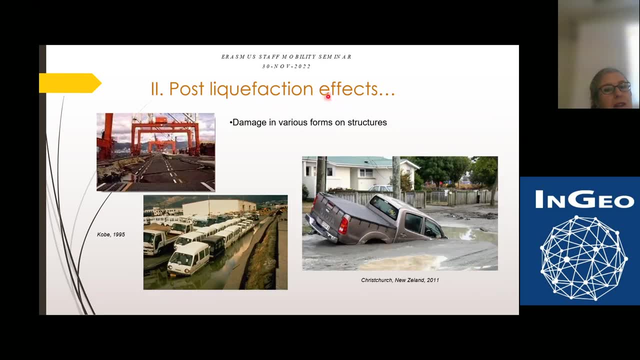 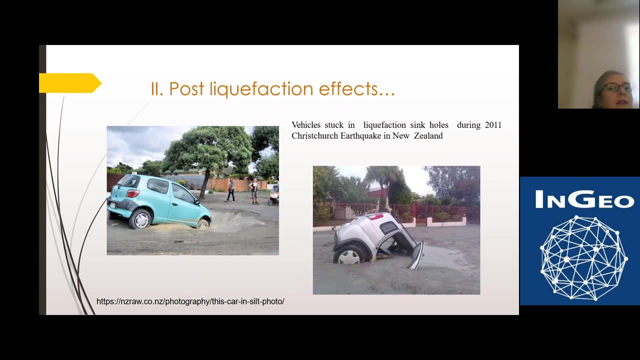 It's a nice, I think, laboratory in nature to have an idea, especially the sand boiling material. Besides, as you can see, with the damage in the various structures within Kobe or again Christchurch, And even some sinkholes that may occur within the whole amount of the material, 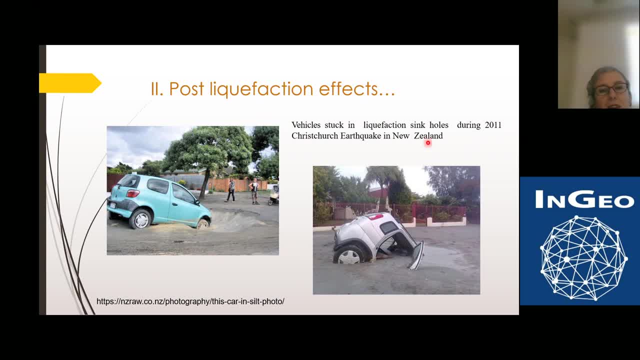 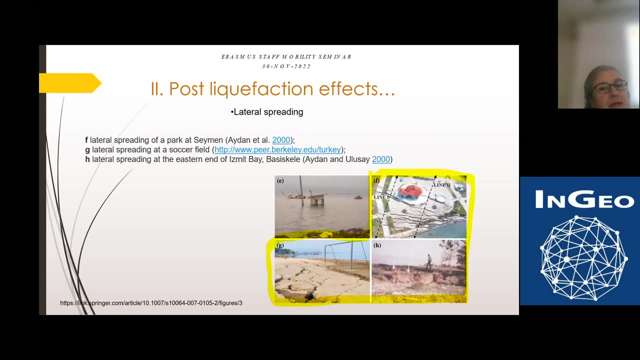 Is the behavior of the liquefaction related? Sorry, I couldn't give some of the important items because I have to keep them for tomorrow. Therefore I need to maybe just give the general idea that you are going to have And again from another view of the lateral spreading. there is also related with the 1999 earthquake. 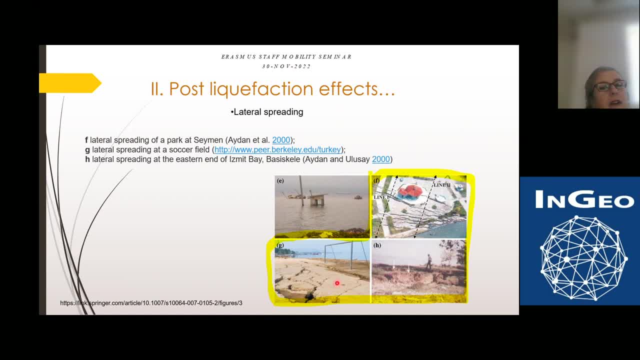 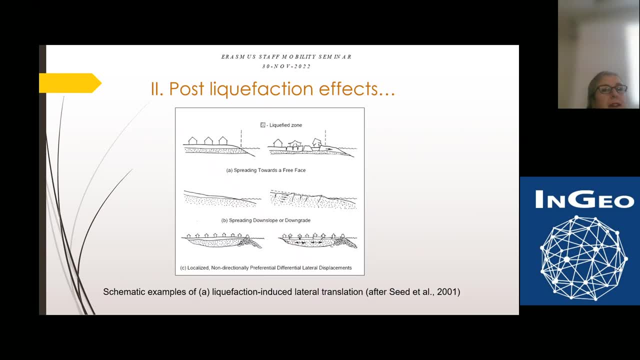 And here you can see the displacements in the park or within the Region that occurred in that area. So For the effects, as I told you, we have a liquefied stone, It's free. And then there are some moments that occurs with the lateral translation that I might say in that sense. 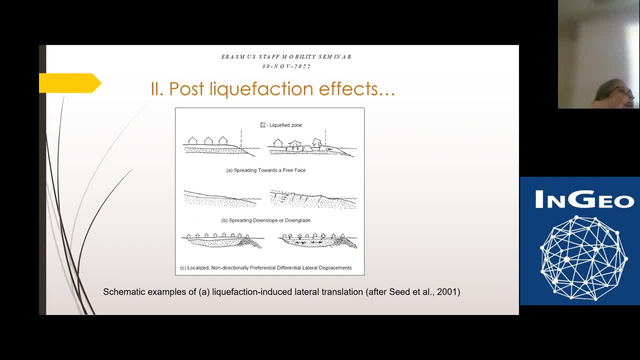 And you can see some schematic examples Why I am putting these examples. I realize that we are theoretically perfect. We can draw everything, But while we are having the experiment or the other things, it's really changed. We cannot see the vertical parts in the fields. 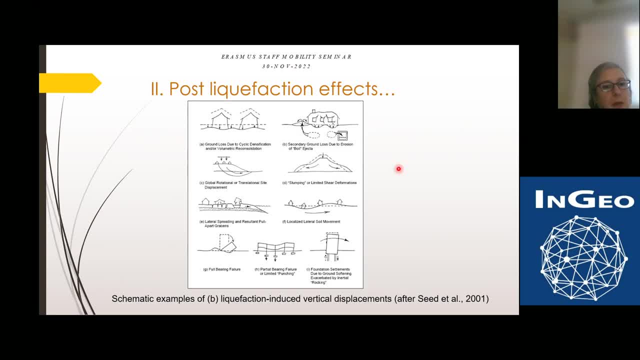 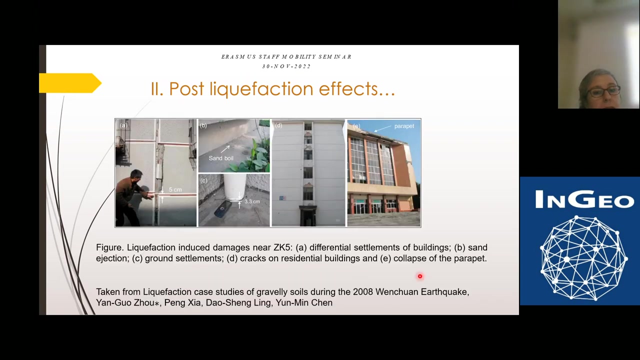 And even with the other type of the behavior, with the vertical displacements, And here you can see the different behavior that occurs, especially in the sense with the lateral spreading Or some bearing failure with the, Actually depending on the foundation settlement And you can see after 2008.. 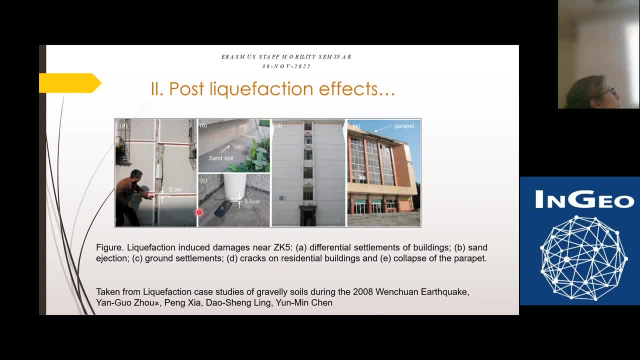 Venture earthquake. There are some Hand boils that comes from a structure. So we need to also consider that there will be a kind of differential settlement or there will be some problems that may occur in the structures. Liquefaction induced problems: Another case. 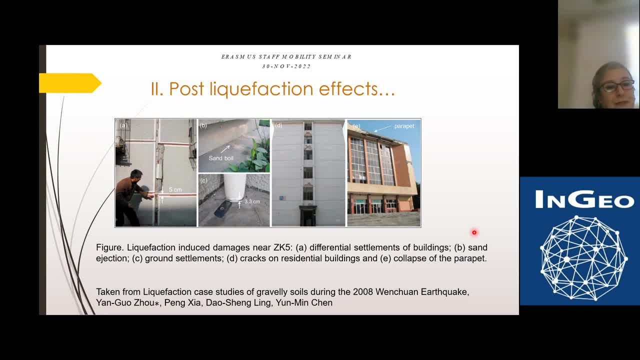 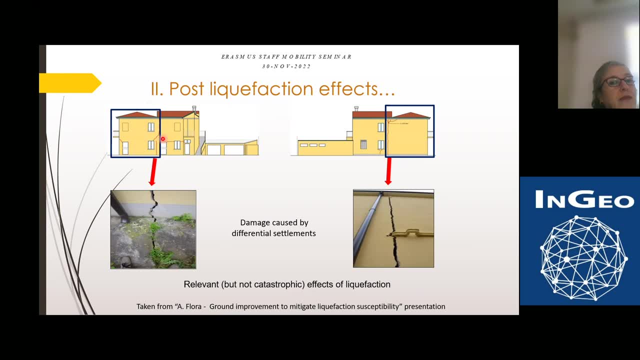 Maybe we should work with the structural engineer And with the, again, differential settlement. it is not catastrophic But, as you can see, there are some adjacent behavior in between the structures. You can observe with the settlement or differential behavior that occurs in the structures. 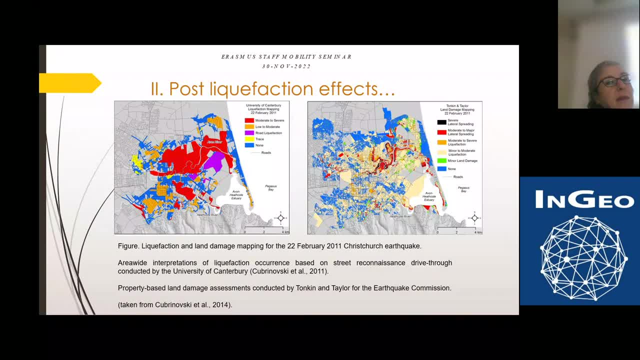 What else I should say: Okay, there are some approaches, We are making some maps, So how we can decide the map is necessary, or how would be the scale of it, Or we should be sure about the details Here you can see. 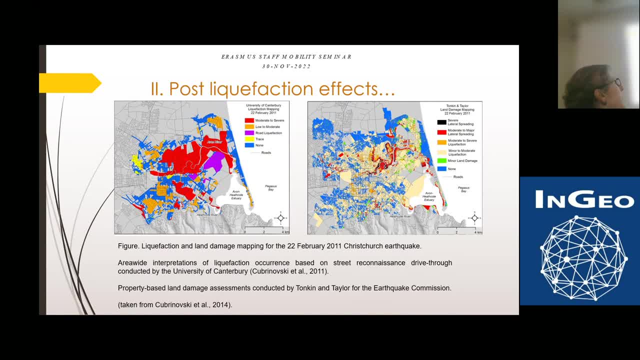 From. They have actually studied Some Places. depending on the liquefaction mapping- or liquefaction, Not the triggering- You have to also consider the hazard index or the size of the liquefaction potential or severity. So it's another issue That I have to say. 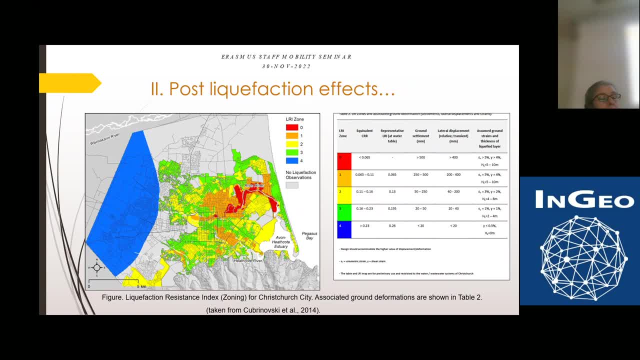 In here. I really like this When I'm seeing that liquefaction resistance index is the kind of maybe index. We should also consider about that, because it's depending on the observation of liquefaction. And here you can see the distribution of each equivalent CRR. 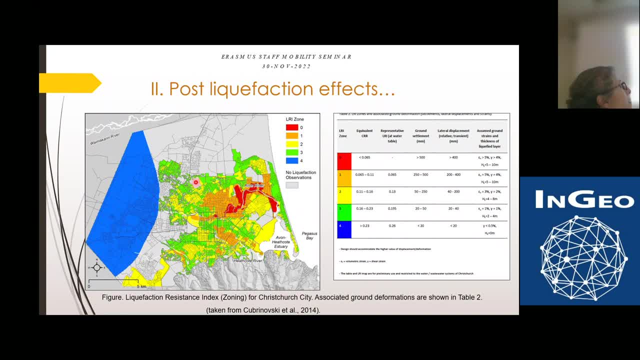 And there are some settlement that may occur in this zones. So it's kind of a microzonation or liquefaction based, I mean, maybe the combination, all of it. So it's another issue that we need to consider, Or, while we are having our microzonation, 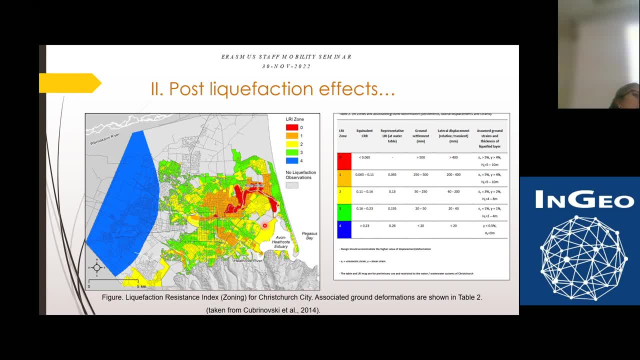 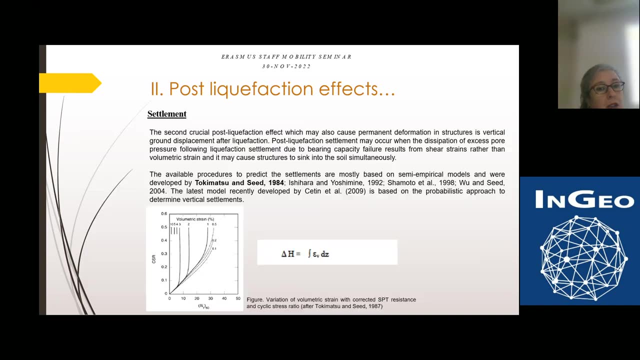 We need to add liquefaction. in that sense, We did a hazard index. It's a good example. So these are the effects that we have seen, But how we can solve, or how are the methodologies? We have actually settlements, As you know. 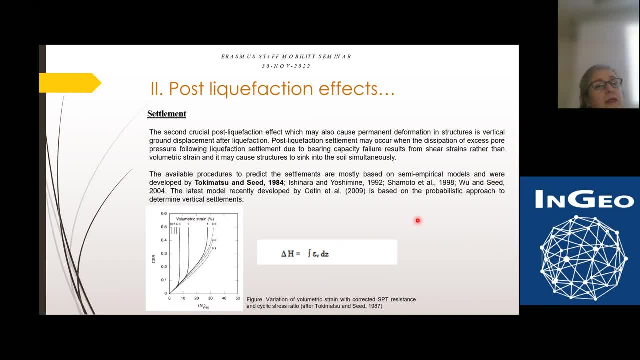 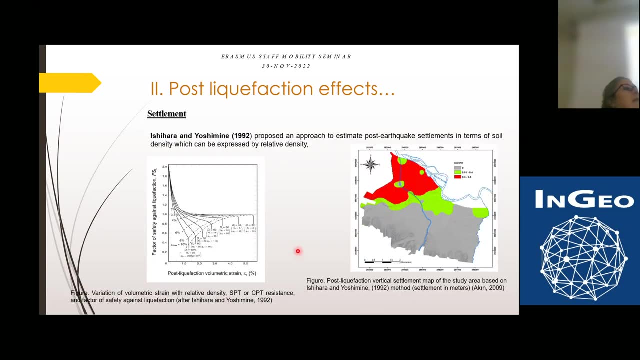 We have different approach Depending on Tokimatsu and seed, Ishiar and Yoshmin Shimamoto and seed And additional databases Additional approach that we are having. I have actually used some of them, By the way. I have studied. 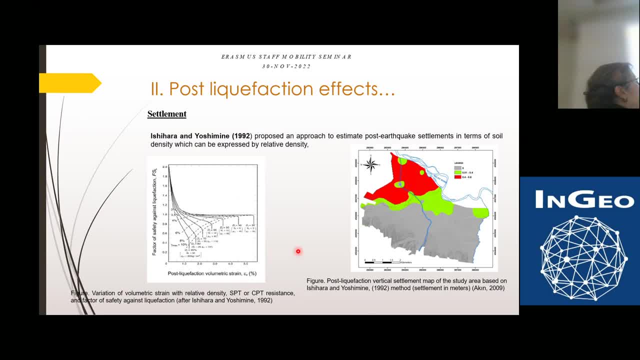 Seismic microzonation For a specific area. Tomorrow I'm going to talk about it a little bit. I have prepared the vertical settlement Depending on different formulas actually- And one of them- Here you can see the area- And then depending on the amount of settlement. 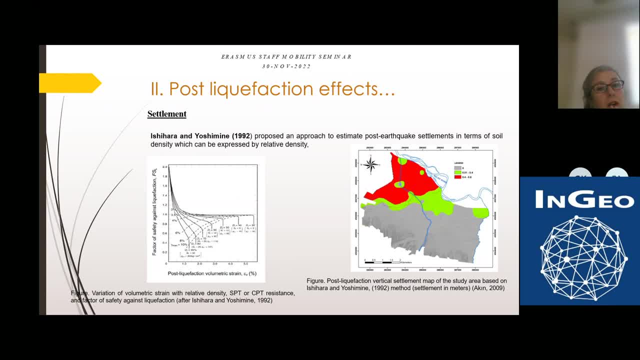 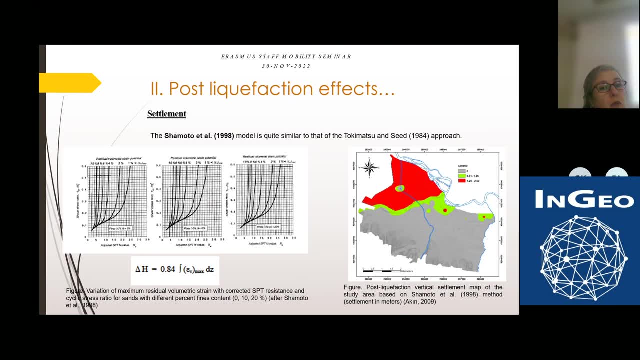 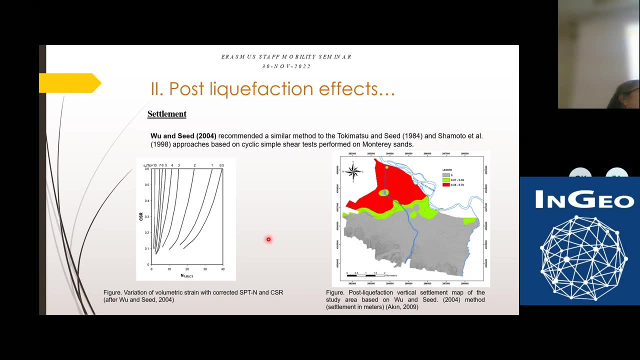 That may occur with the liquefaction Or even with the Shimamoto. I have used Some approach, Depending on the graphs, And with the other one, But another case: Which methodology should I use Or which Amount of settlement should I take? 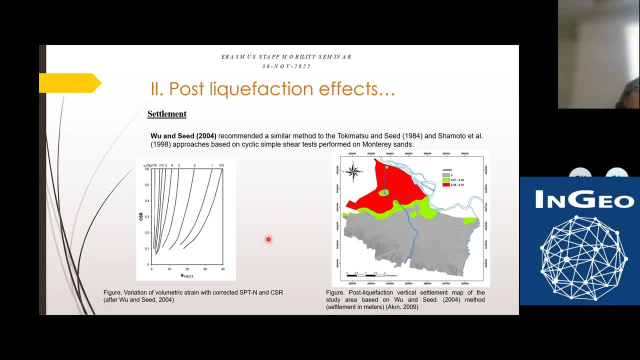 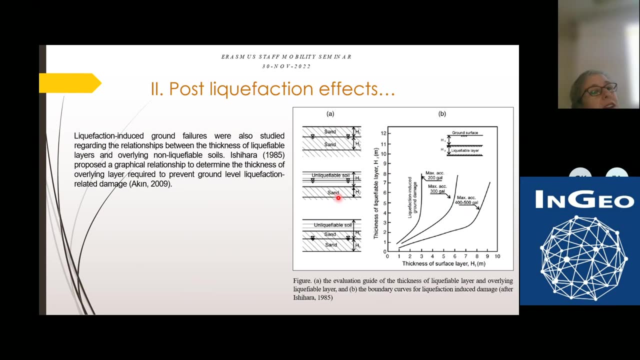 Or even for the lateral spreading, The newest version Or the previous one, Or how can I decide? Another issue, And The thing that I have mentioned also This is the thickness of liquefiable layer And overlying non liquefiable soil. 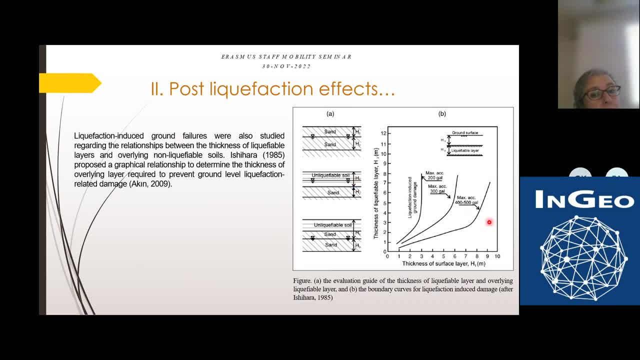 Here you can see Their approach, And there are some curves. Actually, Depending on liquefaction Induced ground damage, Do we need to update this Or are there new updates? Yes, Another thing For the post: liquefaction effects actually. 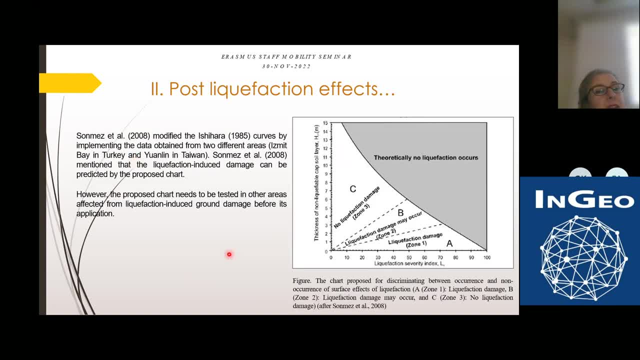 And what else With this? So Some Modified The Curves After The 1999 earthquake And They thought that They have to use, Or we have to, Liquefaction severity index And then we should decide the thickness. 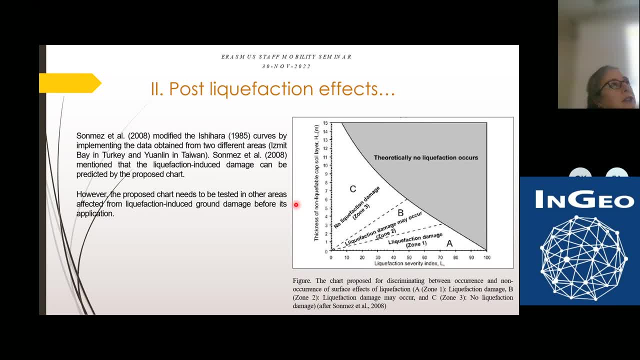 Of the Capsoil Or non liquefiable soil at that stage. This is another item. We need to work on it. There are some still cases Because The proposed chart needs to be tested And, As I Mentioned, 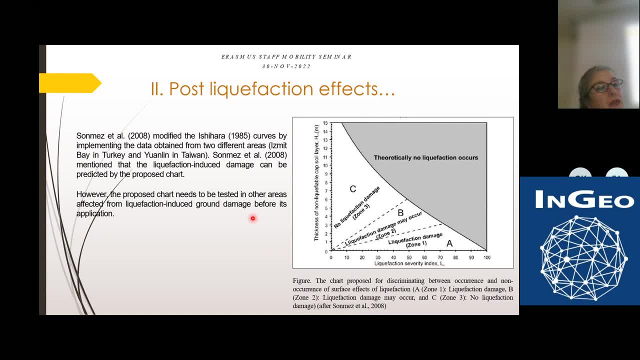 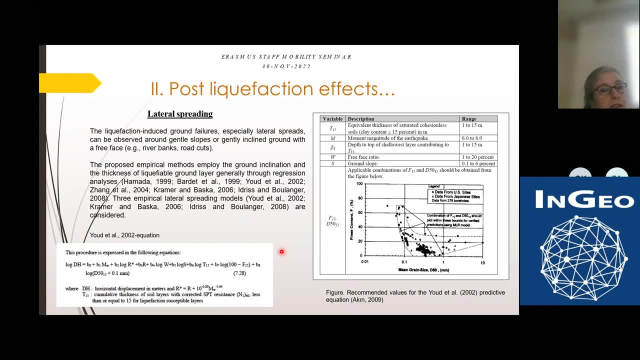 In the Slide. So With the effect of liquefaction Induced Ground damage Before Its application. So It's Another week And For the lateral spreading How we can obtain The results, Or Which. 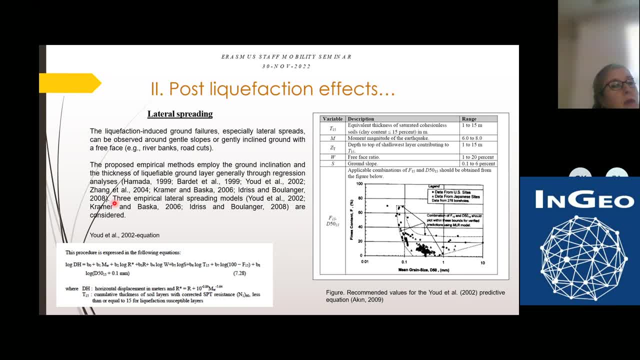 Formulas Should we use In here? As you can see, Some of the researchers Depending On empirical models. That Actually Deals With The behavior, And Maybe We should Add In somehow Sloping. 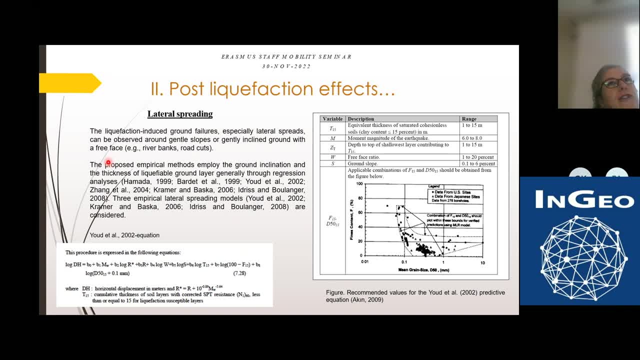 Ground Or Sloping Amount For the Lateral Spreading, As far as I can See, Because We are Having Some Corrections For the Key K Related, As you Remember. 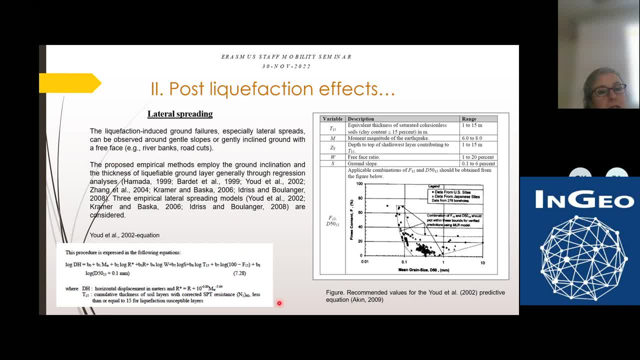 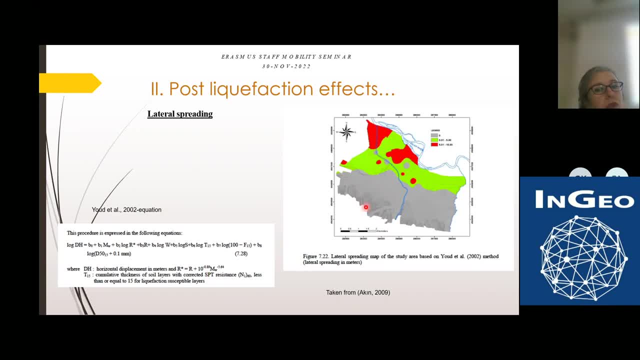 For The Consideration. As far As I Can Understand- And Here You Can See One Of The Approach And You That Whole Equation I Have Used- 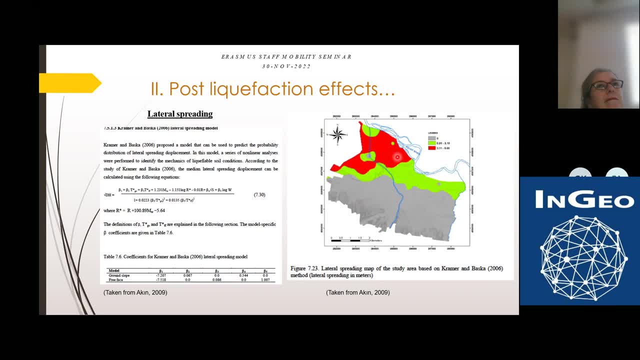 Again Lateral Spreading Amount In Somehow Here Or Bigger. Why? Because Of The Approach Or Because Of The Cases, As You Can See. So 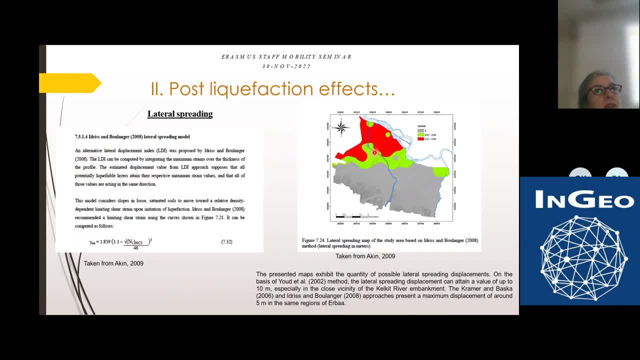 That Would Be Some Comparison, Or We Need To Decide And Lateral Spreading Or Even Settled This Is. We Need To Talk, Maybe, And 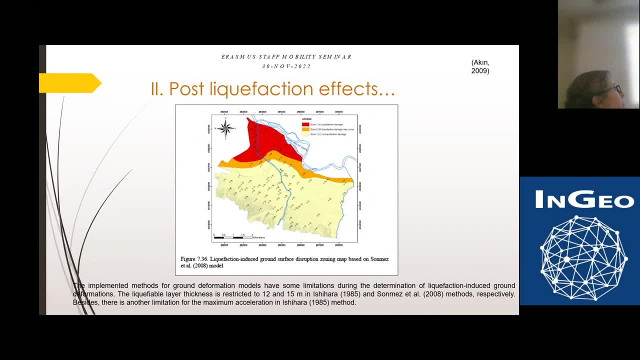 With A Post Occupation Effect, With The Ground Deformation. It's Also Necessary You To Have A Zonation In The System. So This Is Another. 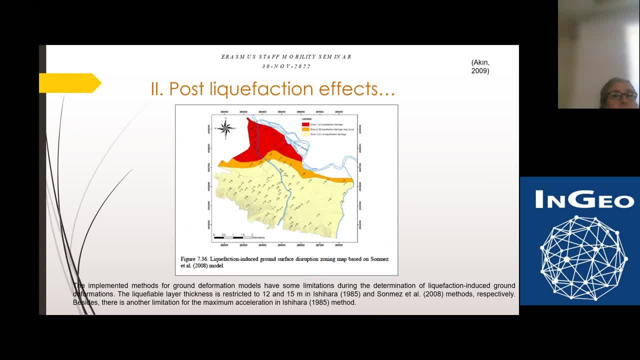 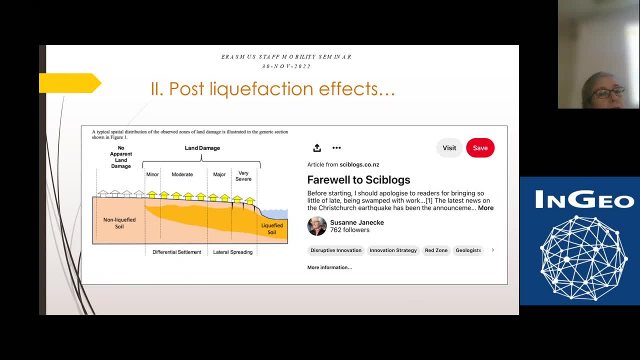 Thing Why We Are Having Acceleration Value Or Why We Are Using Pga Or Magnitude Or Etc, When I Am Finding This Very Severe. 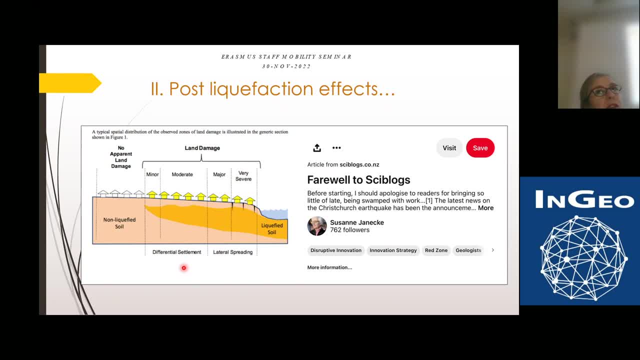 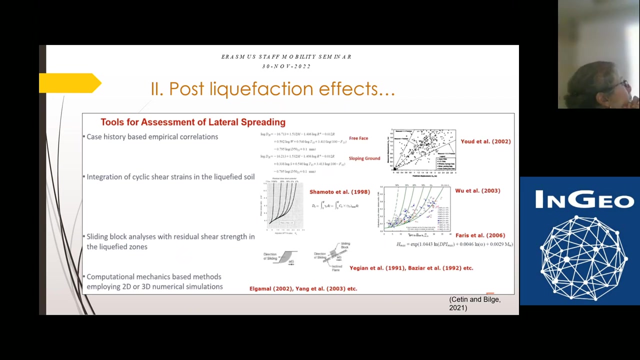 Or Major, But It's Continuous With The Land Damage, With The Differential Settlement, So Maybe We Should Study Both Or At The Same Time Give. 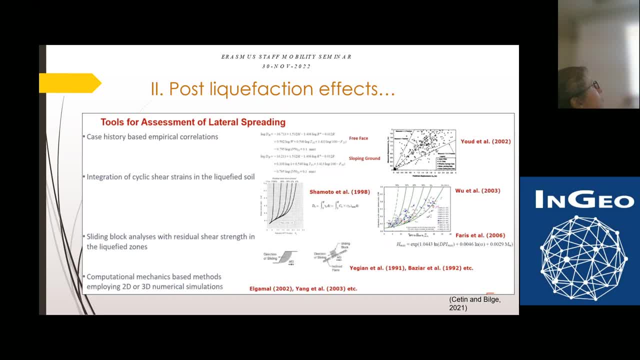 The Similar Chess And Being Divided Into Them Like Empirical Correlations Or Integration Of The Laboratory Work That They Have Or The Other Researchers. 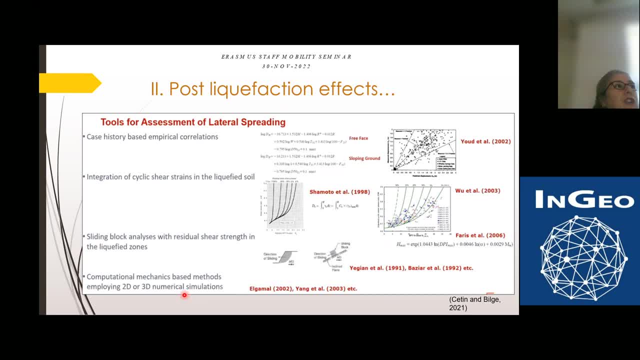 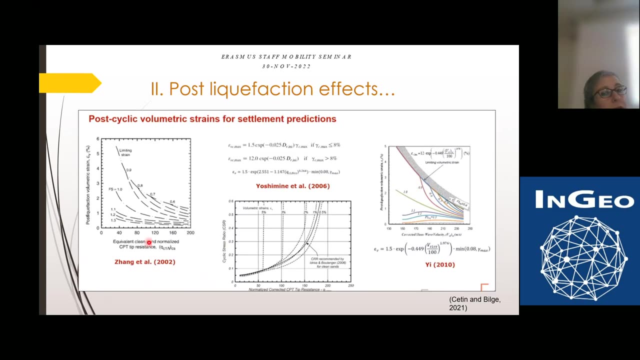 Have Or Some Sliding Block Analysis, Or These Techniques, And These Are The Latest Versions, Even With, Again, Settlement Predictions. We Have Another Approach Like 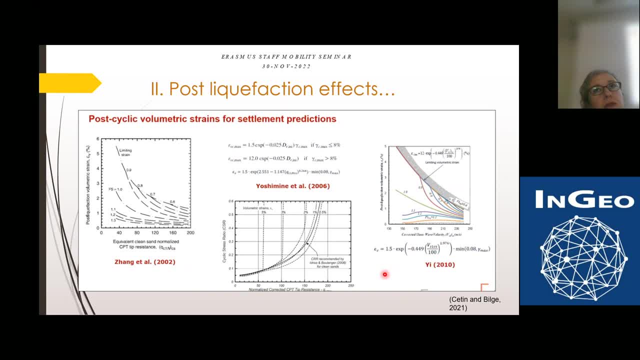 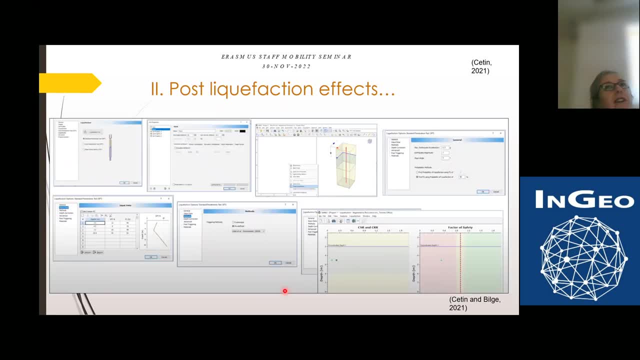 You Or Your Spin. These Are The New Generated Curves And The Spheres. I Don't Know Which One Is Famous. In Italy We Have 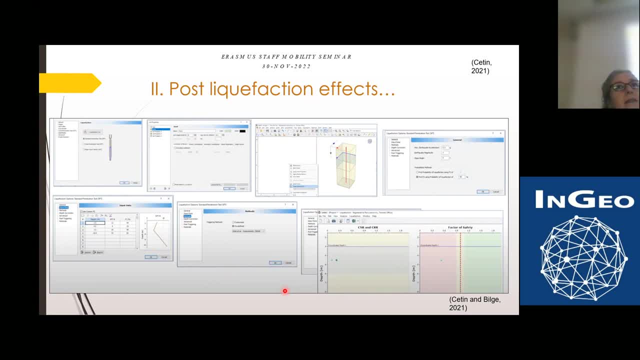 Rock Science Programs Generally Saddle Or Slide Or Etc Or Geo Five, I Heard, Or Even Plexus. We Are In The Settlement We Have. 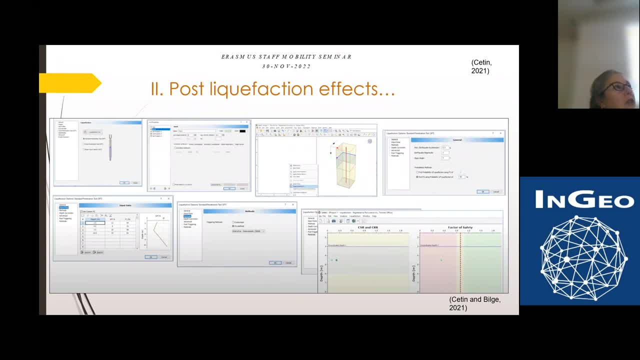 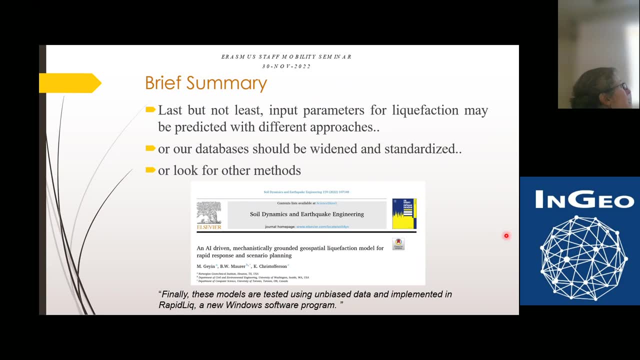 Some Questions About Mine, Depending On The Liquefaction Related Issues That Before That I Would Like To Say. Last But Not List, The And We. 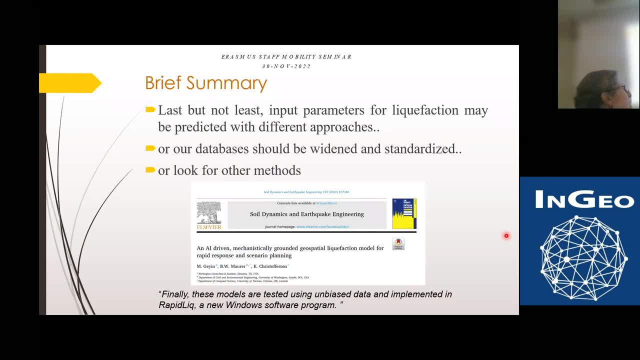 Need To Look For Other Methods, Such As You Can See. It's Just Newly Published- Depending On, Especially For New Students Or New Generation Artificial. 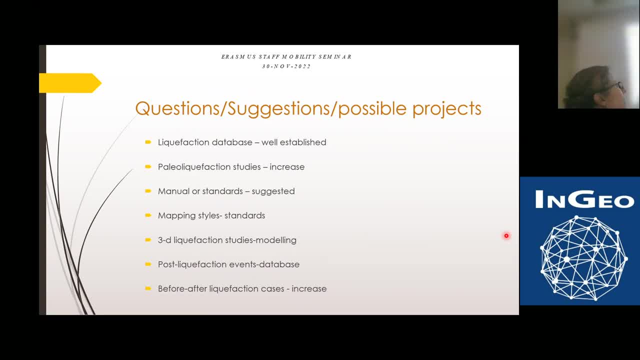 Intelligent Model, And Here You Can See Some- Maybe I Can Say- Questions, Suggestions Or Some Possible Projects, But In This Sense, As I've Said,